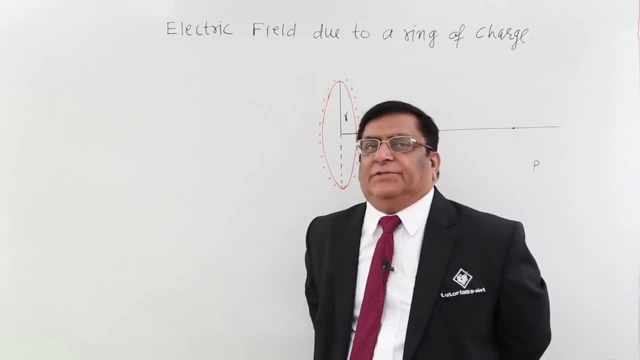 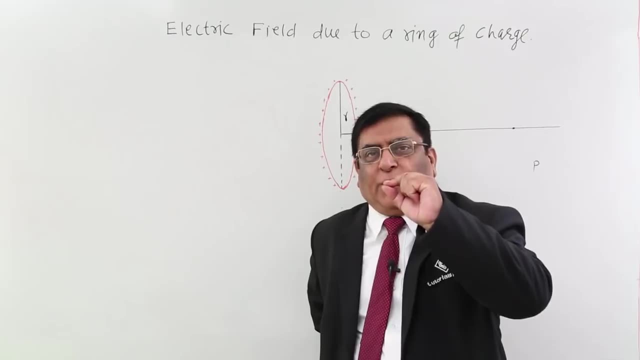 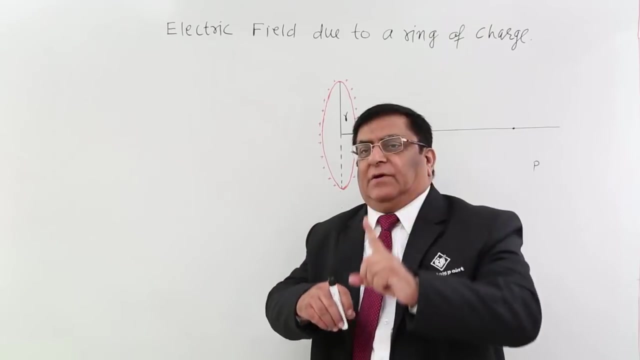 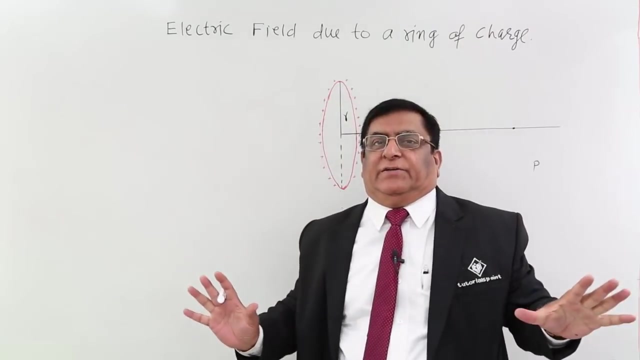 We have done electric field due to different charge distributions. First charge distribution was a charged particle which is a point size. Then we did: the charges are distributed in a very long straight line. how will be the electric field at certain distance? Then we did: if there is one full sheet, very large sheet, in which charges are distributed, then 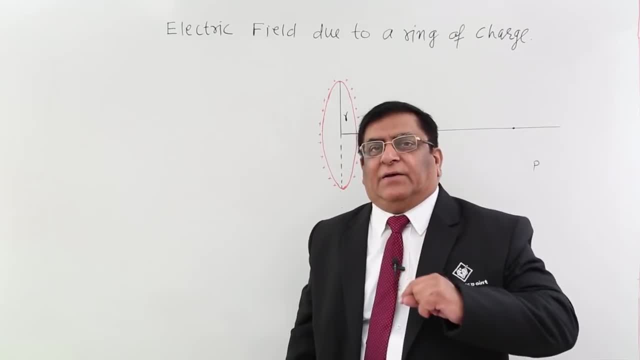 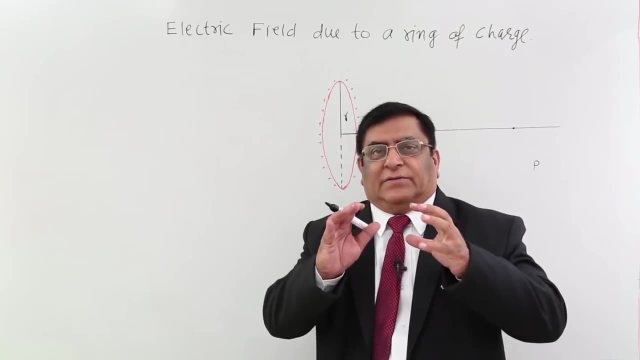 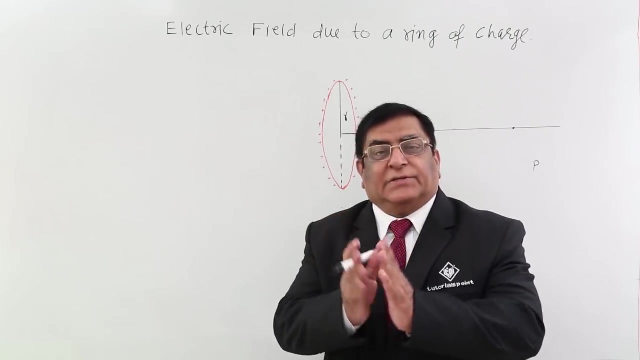 what is the expression for electric field? And after that, studying the Gauss theorem, we got many things like charges inside a spherical shell, outside a spherical shell, inside a sphere, double sheets and many other things. We have also done another charge distribution that is known as dipole, which is positive, negative, both charges placed at certain distance. 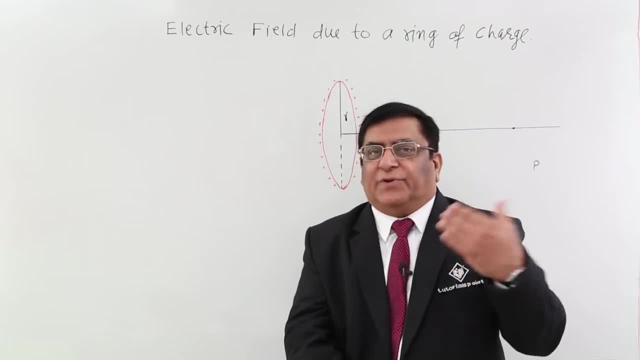 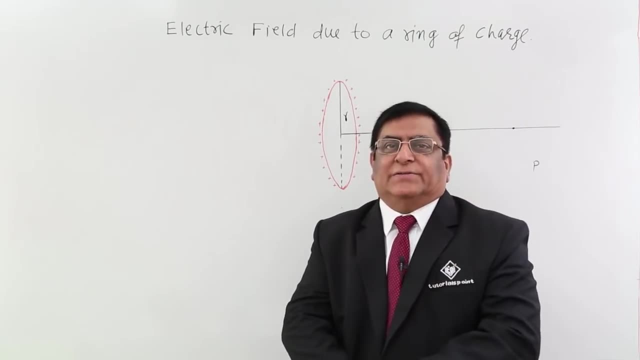 And because of that, how much is the electric field? that is also we have done. Now we will do one more thing, which is again important. it has its own importance and we get such shapes, and that shape is if there is a ring of charge. Ring of charge means we have a. 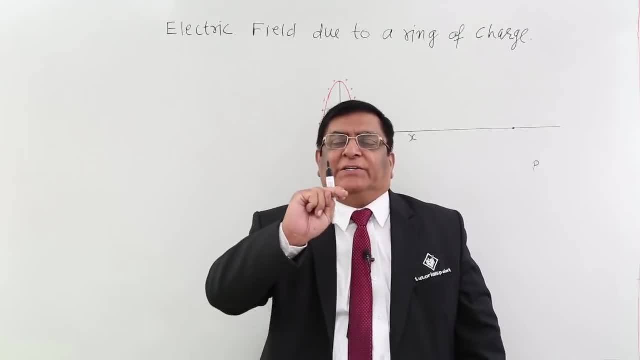 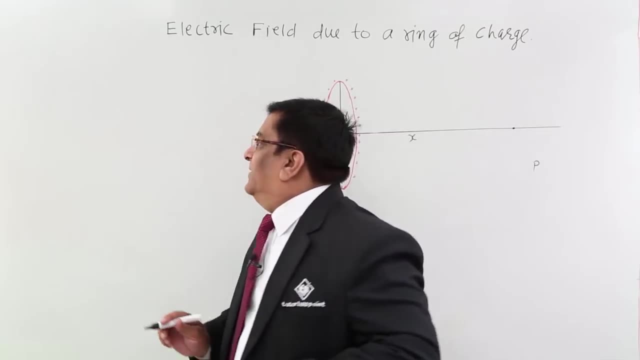 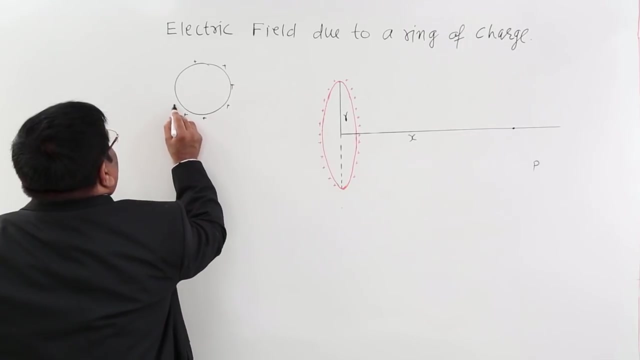 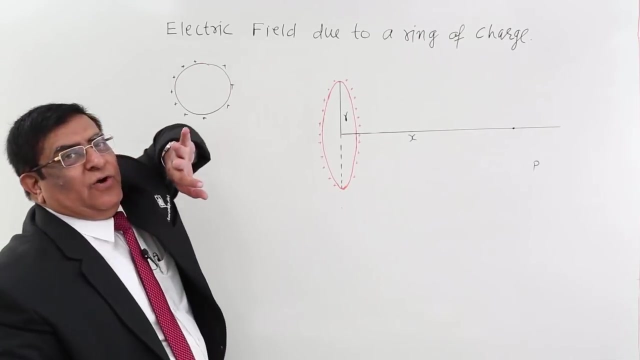 metal ring and we give it a charge. So charge is distributed all over the ring. So where do we work? want to find out electric field. If this is a ring and we make a charge, the charge is distributed automatically on the complete ring. and can you tell me what type of charge? 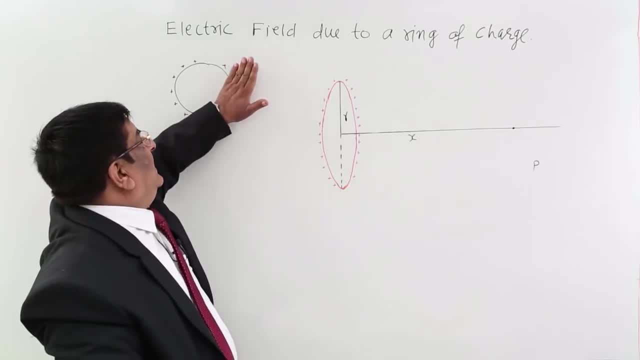 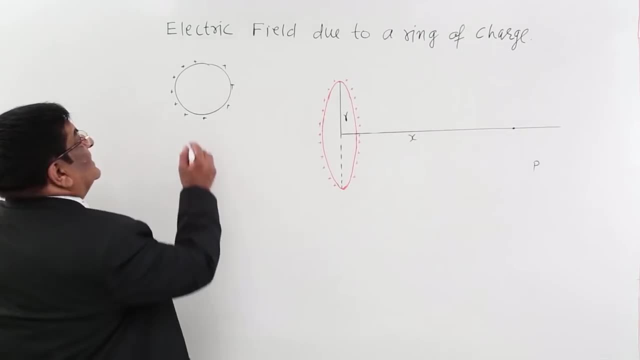 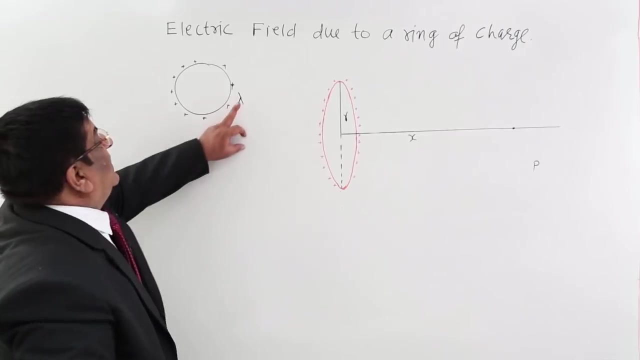 distribution is this: The ring has an area, but no, the charge is distributed on the length of the ring. So this is a linear charge distribution and this linear charge distribution we will denote by lambda, That is, lambda charges per unit length. That is our distribution of charge. 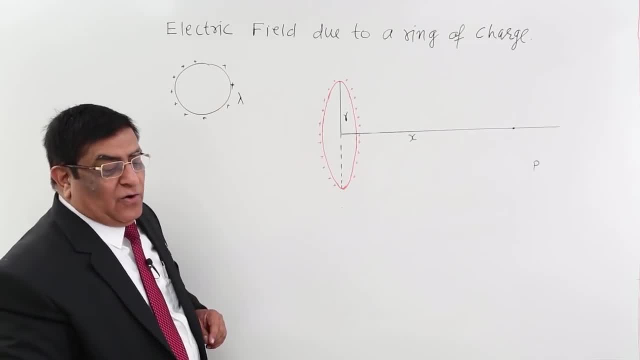 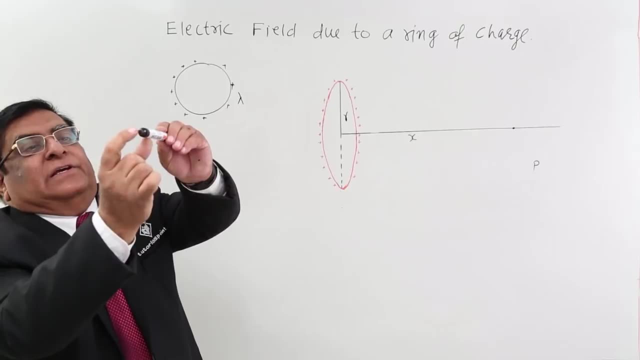 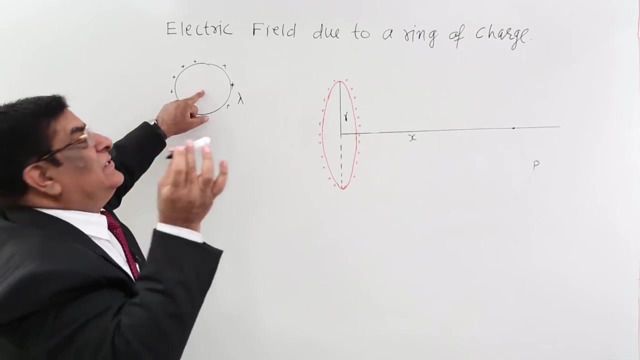 over a ring. We want to find out electric field on its axial line. This is the axial line. I want to find out electric field here at this point. Where is this point? On the axis of the ring? On the axis of this ring And the charge is not in a straight line. This point is little. 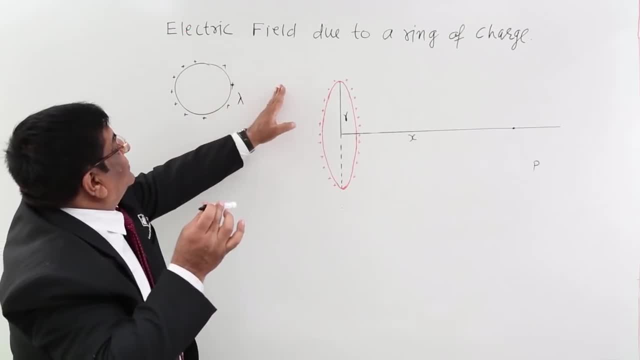 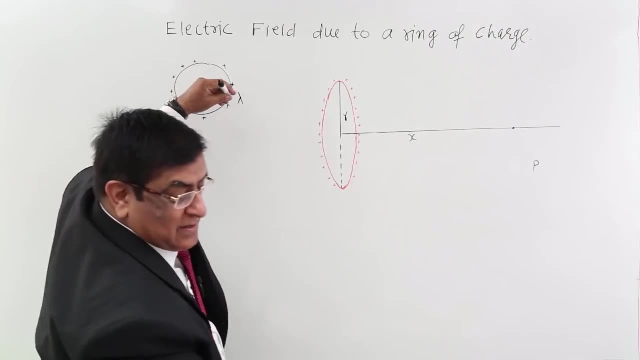 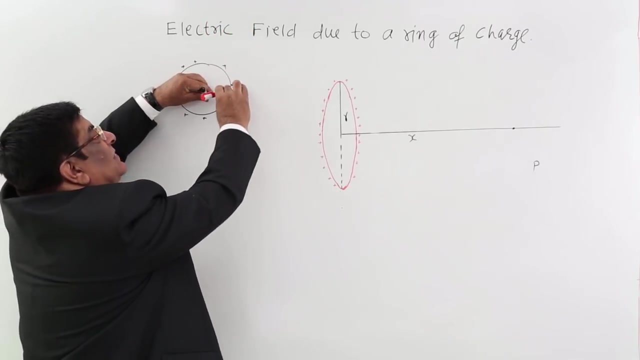 away up. this point is down, this point is right, this point is left. and I want electric field here. This will make electric field in a particular direction. This direction, This will make electric field in this direction. and these are vector quantities, So their 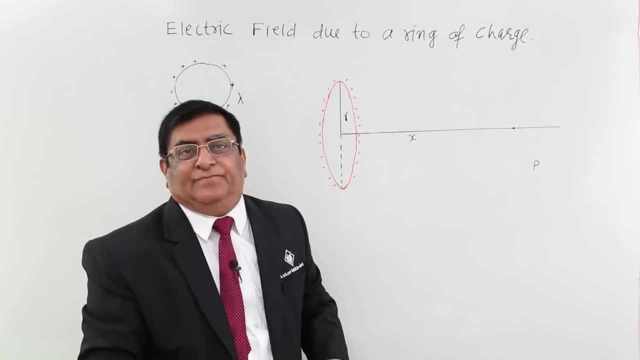 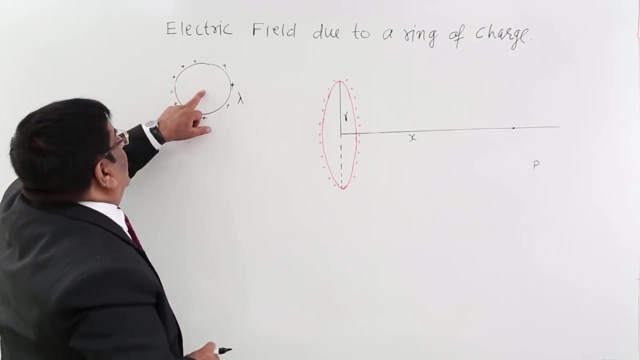 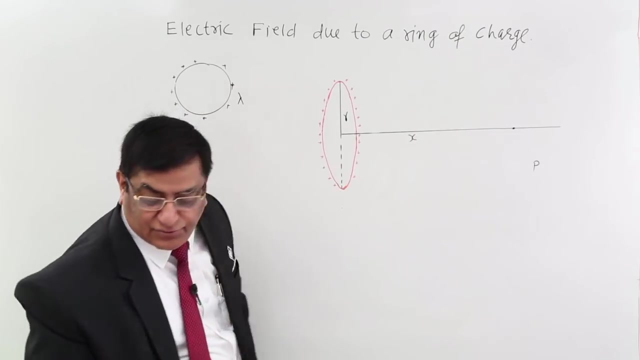 addition will give us a complicated result. Therefore it is not so simple like a point charge. Now I want to find out a calculation. electric field at the axis of a charge ring and its centre is of course part of an axis. So I will add into this electric field due to a ring of charge on a point. So this is: 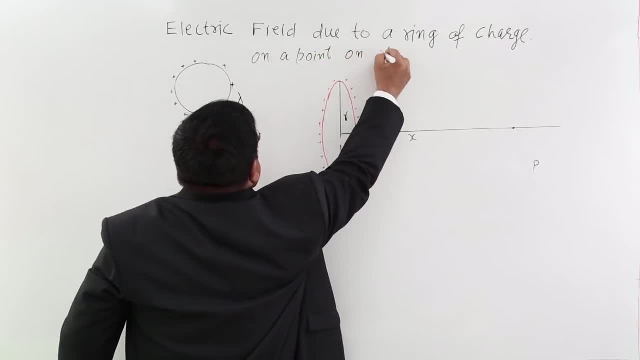 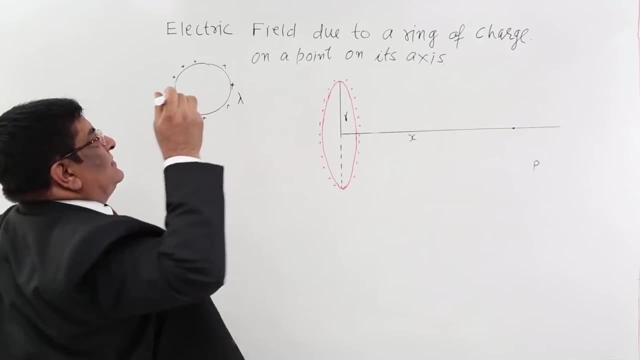 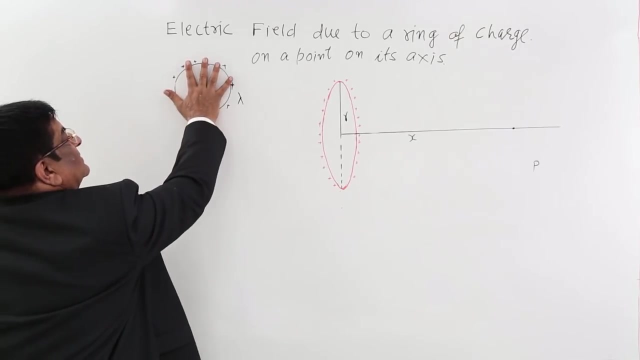 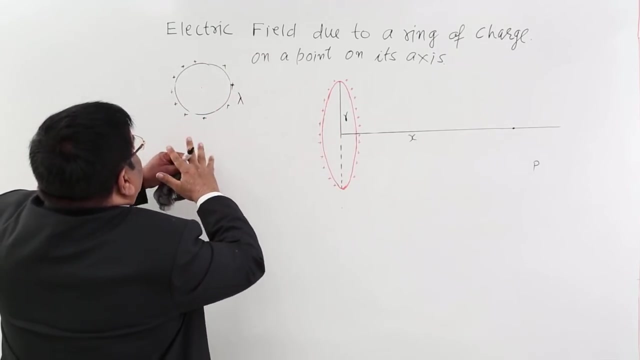 a ring of charge. I does not give you the onion ring, this big track. Then what will I get? All of them, All of them, All of them could be马, All of them could be. Years ago, bribery were exist Right. 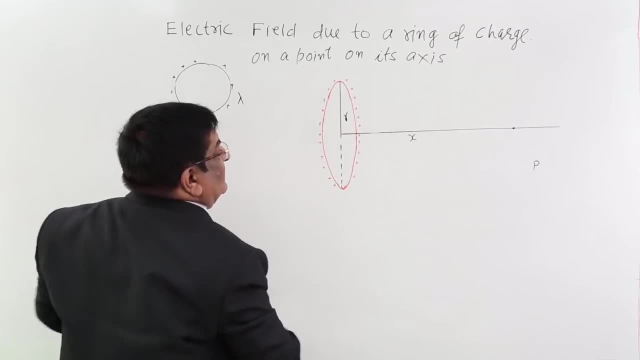 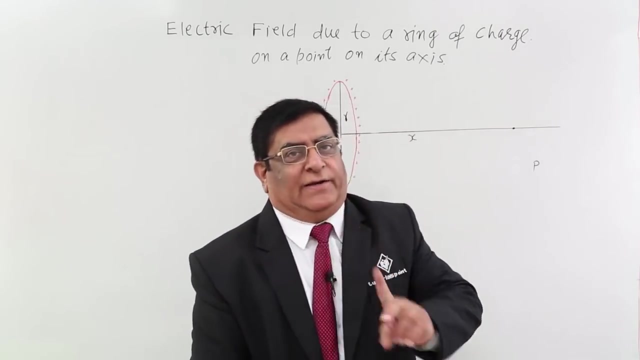 Martinpreneur, etc. So this is the ring, this is the axis. there is a point P on the axis and we are supposed to find out electric field at this point P. Let us start calculation. We know we have only one formula for electric field, that is 1 upon 4 pi, epsilon, 0, Q upon R square, which. 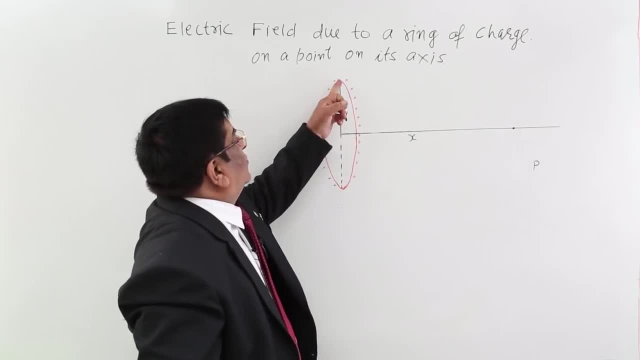 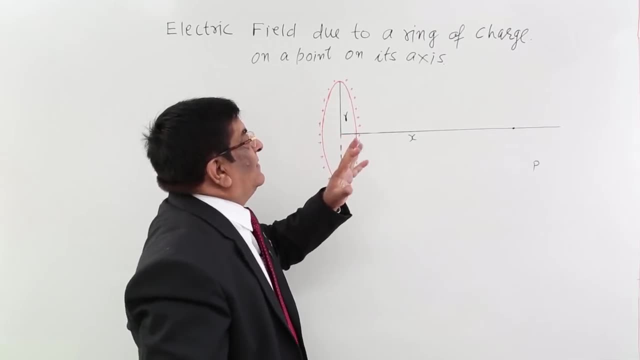 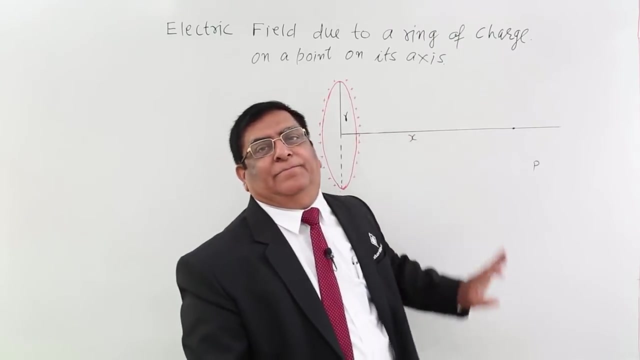 is with respect to the source charge Here. this is the source charge. this is the source charge. There is no source charge here. So who will make the electric field? All these will make electric field and the total net electric will be some of them. So we will. 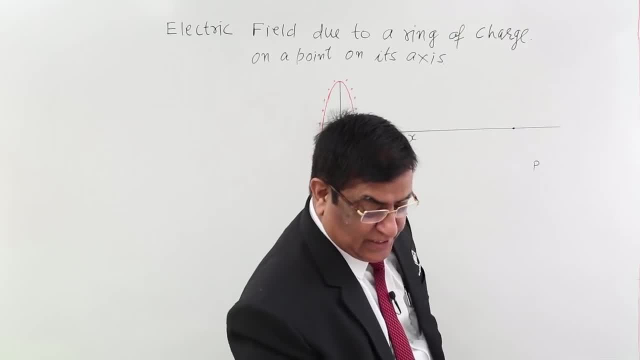 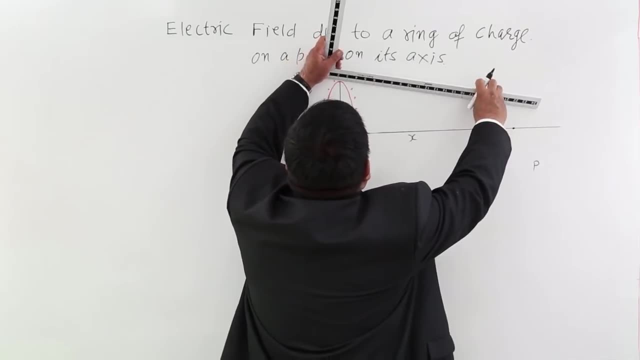 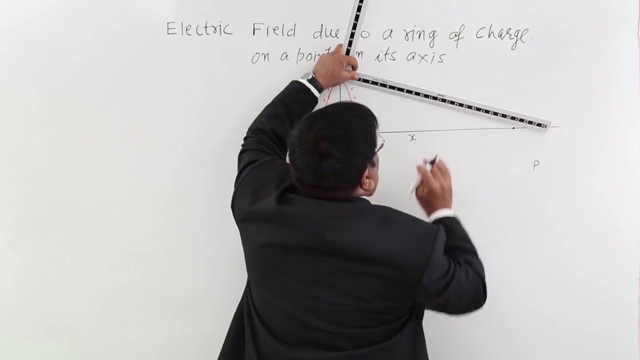 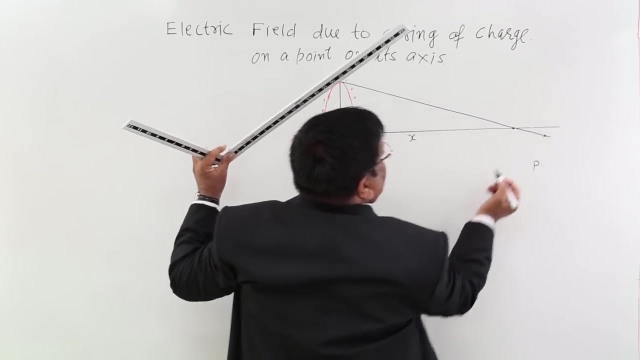 work on this strategy, How we will work on that strategy. See, this charge will make an electric field. in which direction? The answer is: in which direction? This will make an electric charge in this direction, let us say in this direction. 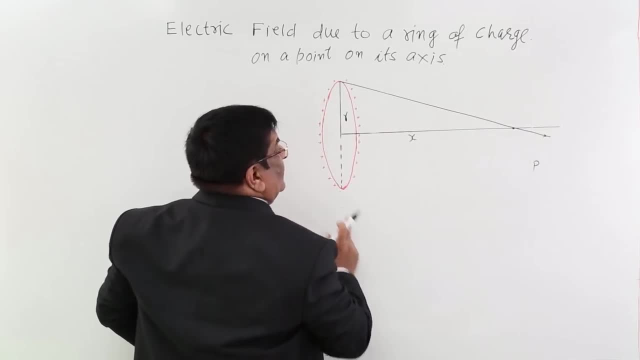 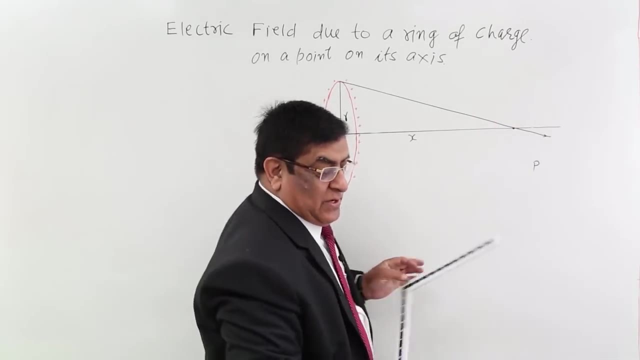 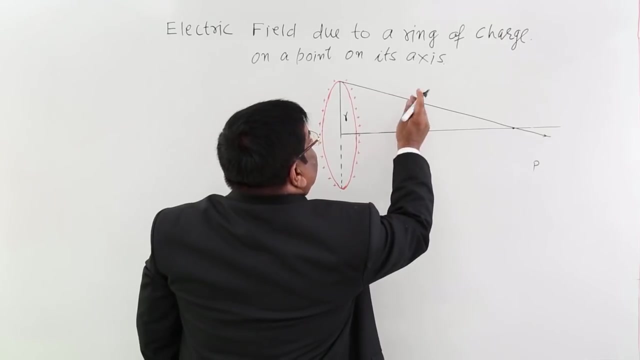 This is electric field made by this charge. but this charge will make an electric field in this direction. This will make in this direction, going inside. How much will be this electric field here? Let us suppose this distance. how much is this distance? So, according to Pythagoras, this is r square plus x square. 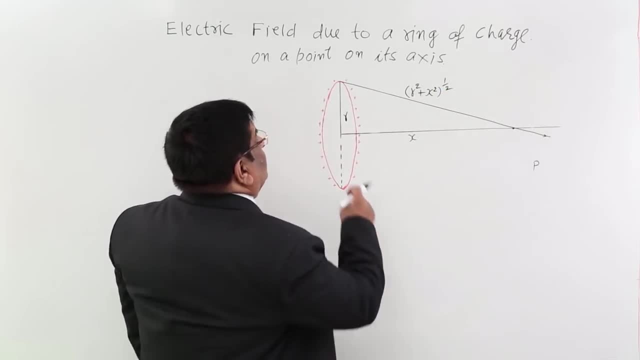 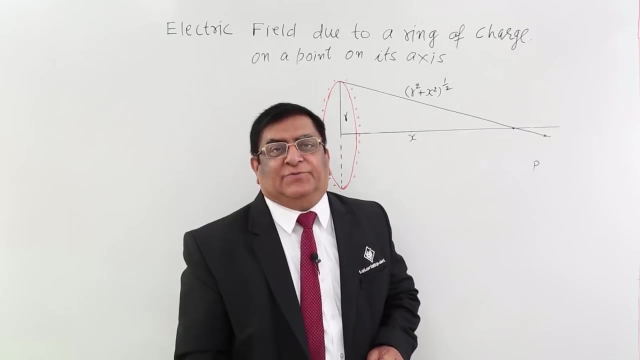 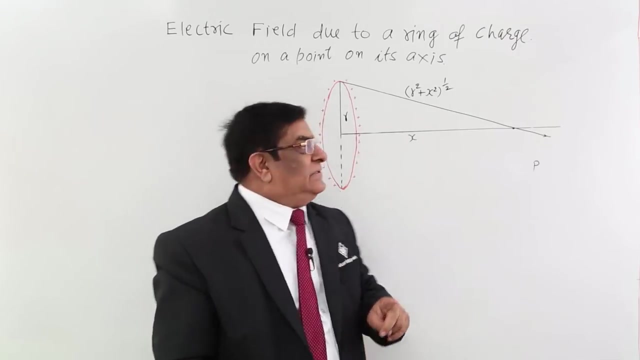 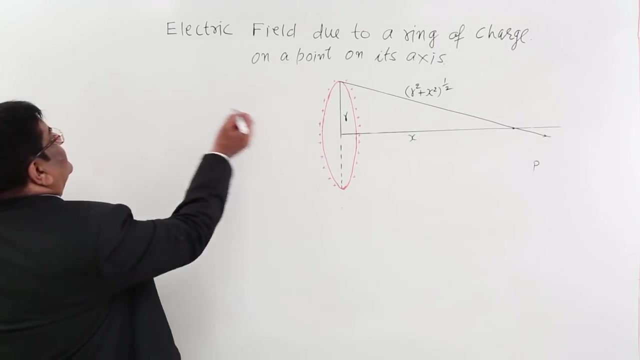 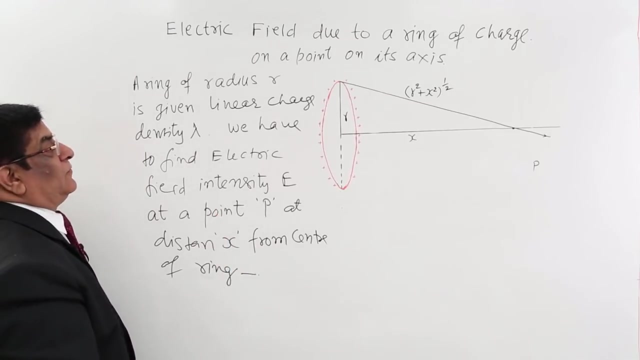 This is the length. Now, here the electric charge is distributed and we have to give certain quantities in terms of which we are supposed to find out electric field. After all, what is given? Two things are given to us. This ring has got radius r and the charge we have given to it is lambda. 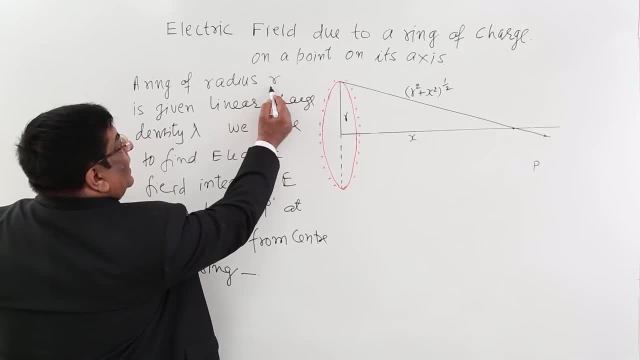 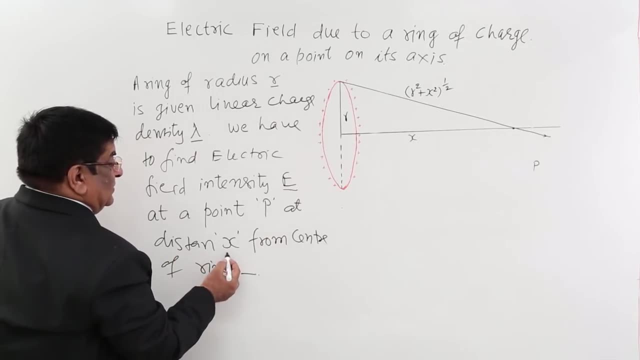 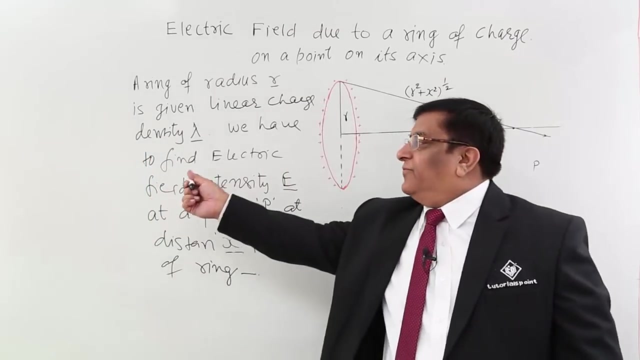 This is the given situation. So we have r, one quantity, lambda one quantity. We have to find electric field, and the distance given is x, The rest formula, epsilon, not. that is already known to us. So we have to find out electric field in these formats. 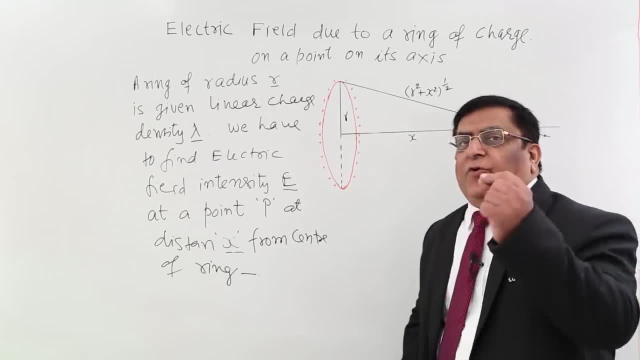 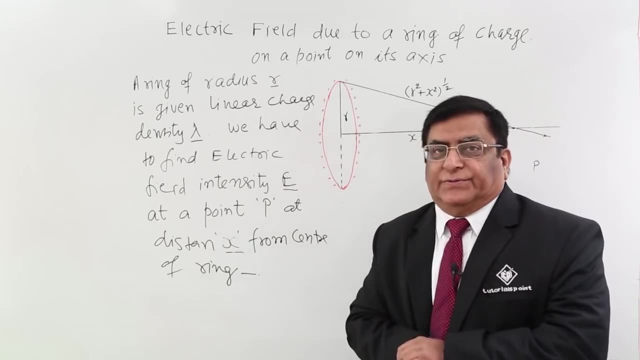 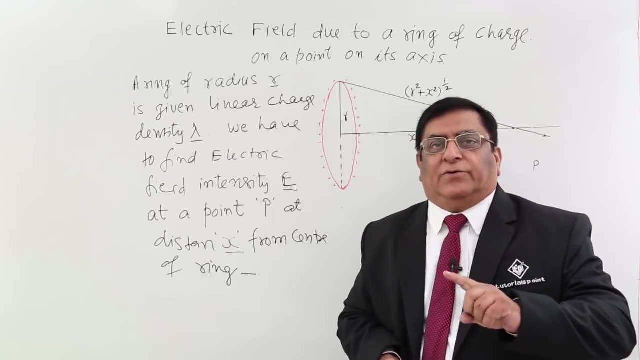 Start it Here. we know the formula for point charge. Here we have length, What we will use. First we will convert a very small length, just like a point, and so far you have learnt that whenever we want to convert a bigger thing into a bigger thing, 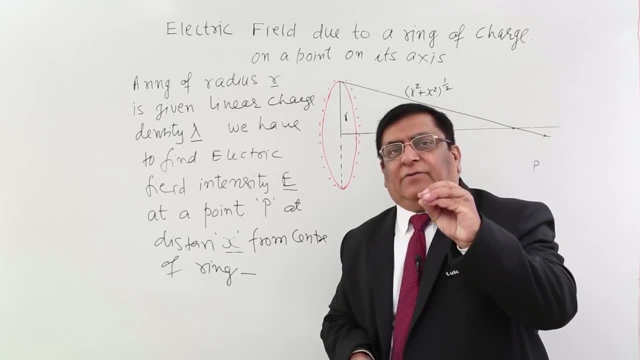 So we have to convert a very small length, just like a point. And so far you have learnt that whenever we want to convert a bigger thing into a bigger, into a point, we take help of calculus. so we take a very small length here: dl, dl is so 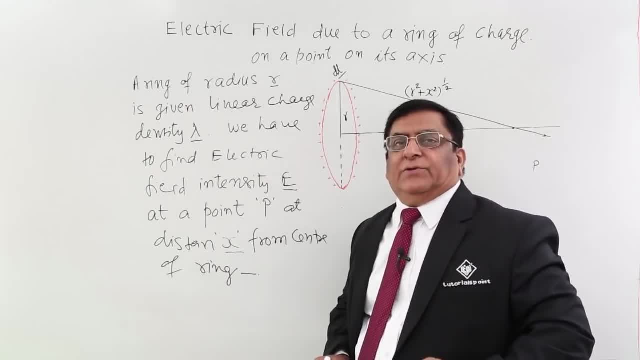 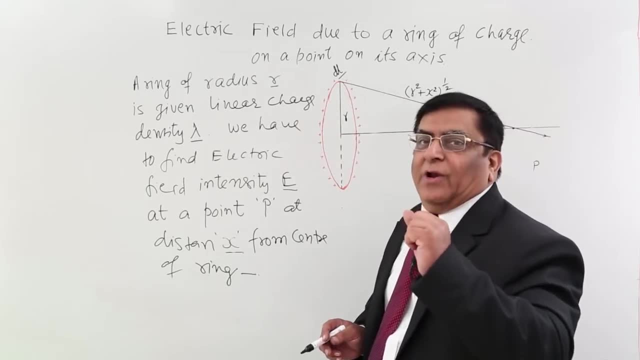 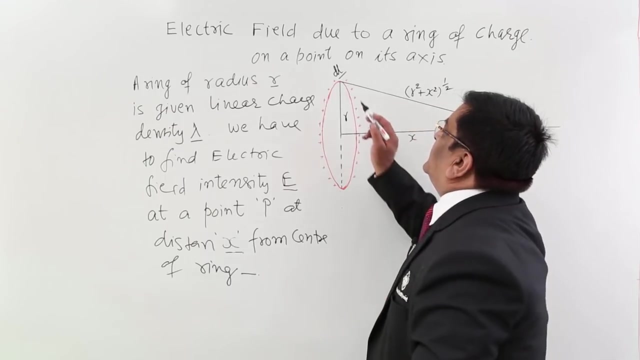 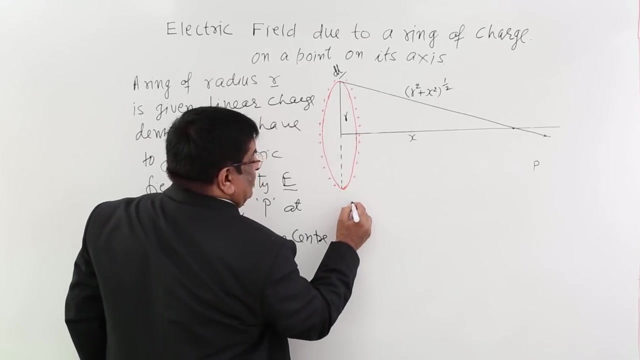 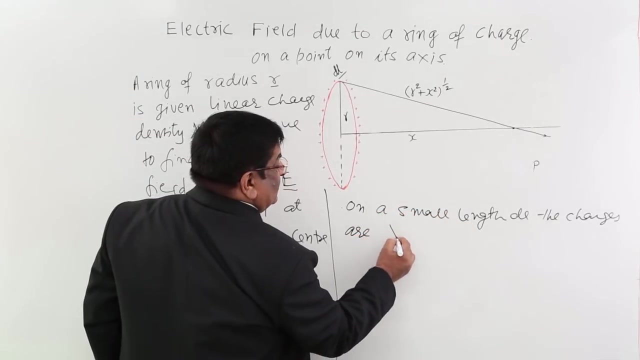 small that it can be treated as a point. so we are permitted to use formula for point if our length is dl very small. so for that permission we take dl. ok, so dl is the length. now what will be the charge over this? on dl, I will write here, on a small length, the charges. 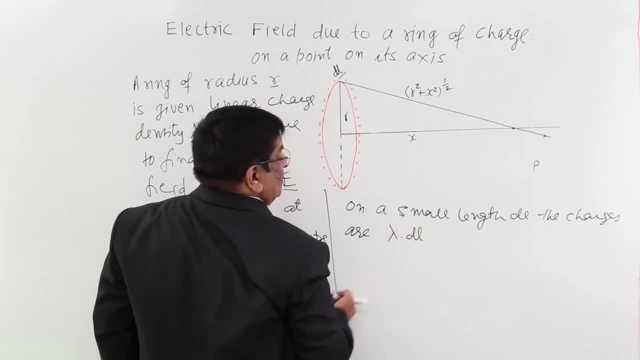 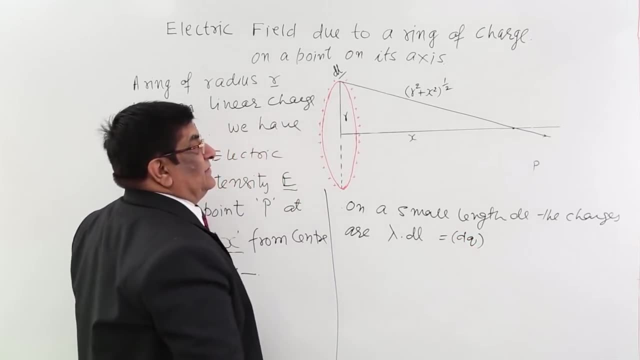 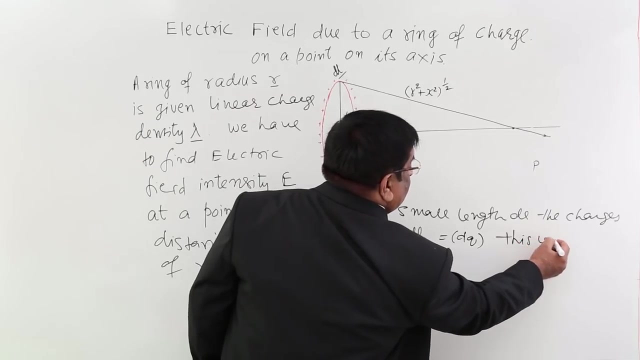 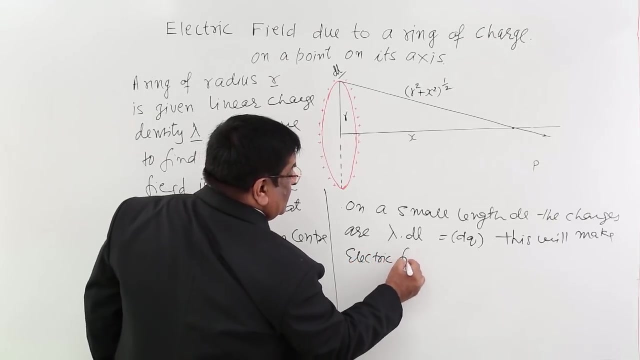 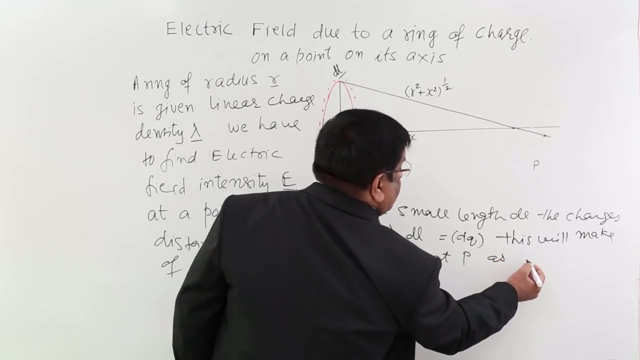 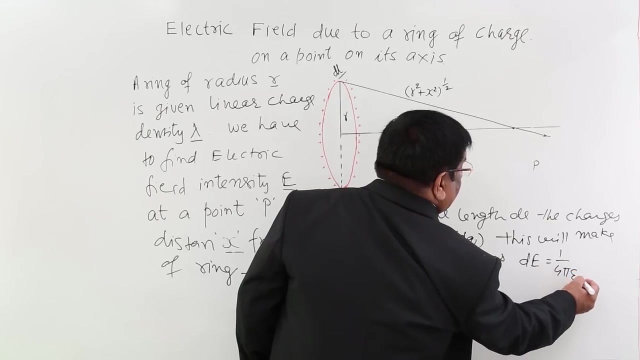 are lambda into dl. ok, now this is. we can term it as small charge dq. this charge will make certain electric field Here. this will make electric field at p as a very small electric field, De which is equal to in magnitude 1 upon 4 pi, epsilon knot dq upon r square. 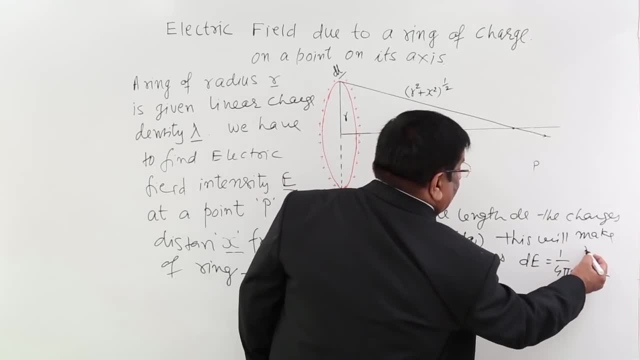 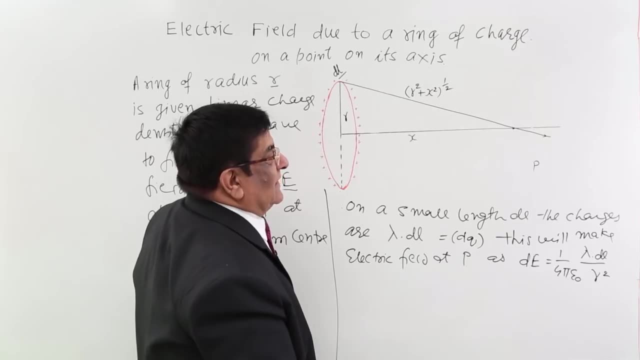 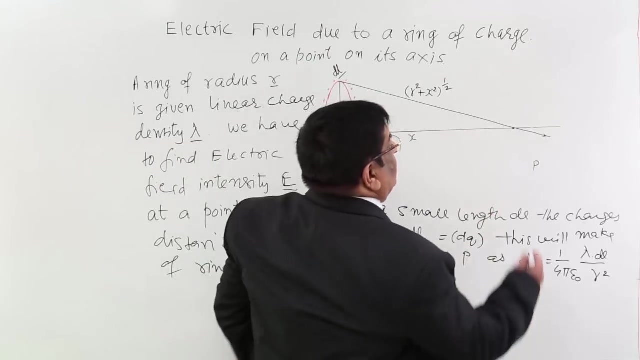 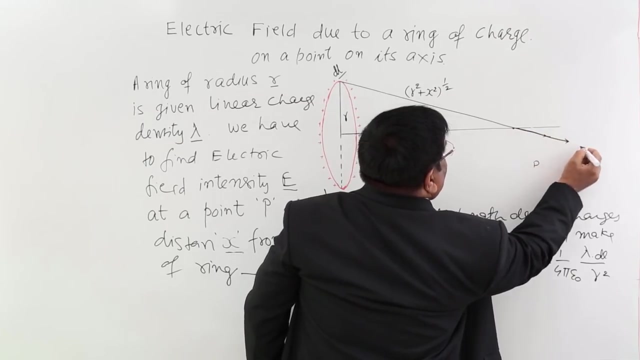 and dq upon dp. we will write as lambda dl. This is the electric field it makes And what is the direction of this electric field? Answer: direction of this electric field is along the line joining the two. So this is the direction of electric field. I will mark it again here. This is: 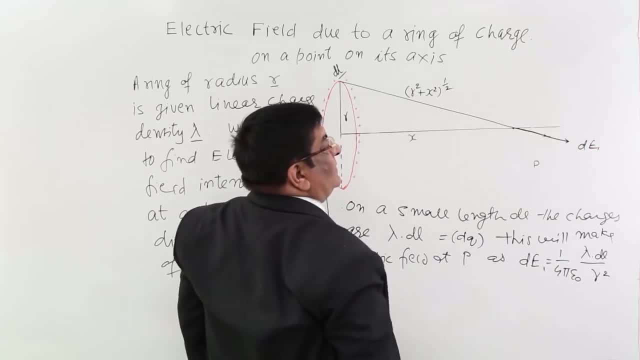 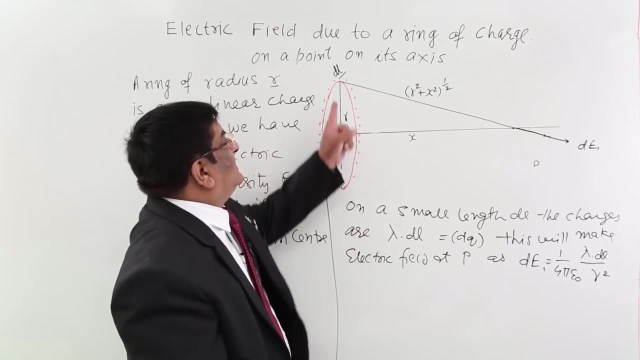 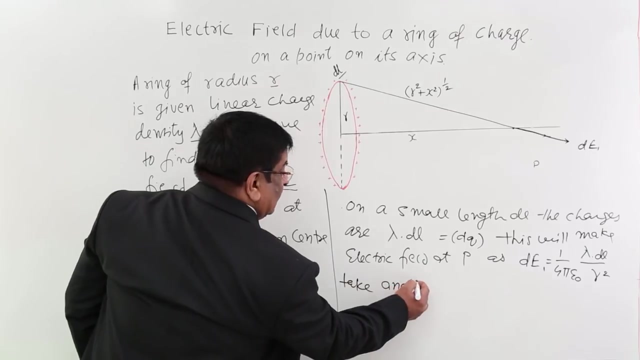 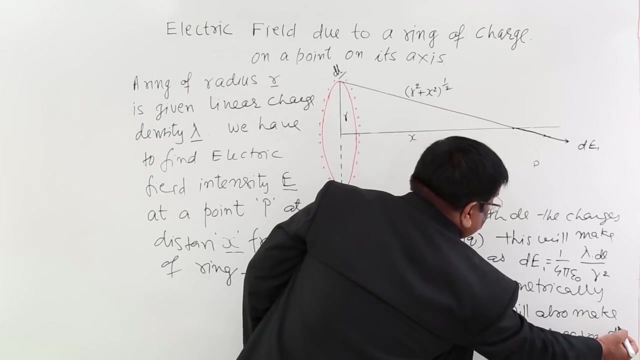 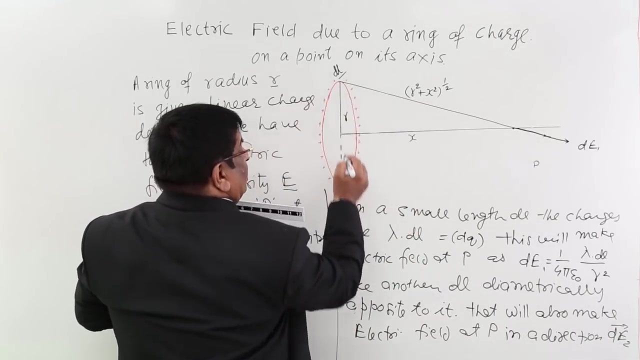 de1 in this direction. Now I take another dl which is diametrically opposite to this. Take another dl, de2.. Where is this de2?? So I take the dl which is diametrically opposite to this. This is another small length dl. How much. 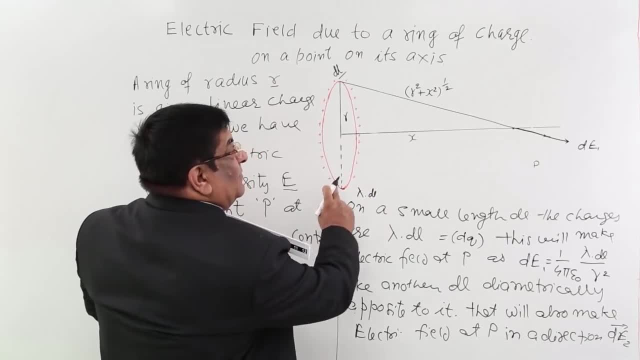 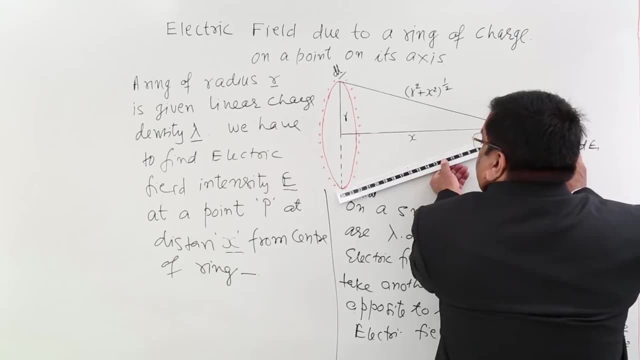 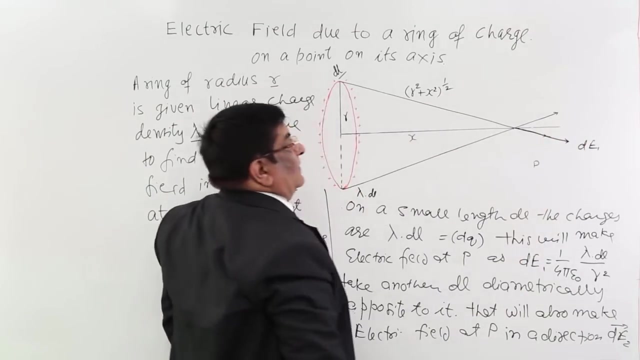 will be the charges in it, Lambda dl. This lambda dl will create electric field here. In what direction? So I put a line here. That line will give the direction of electric field at this point. This is the electric field. Now you know. these two distances are same. 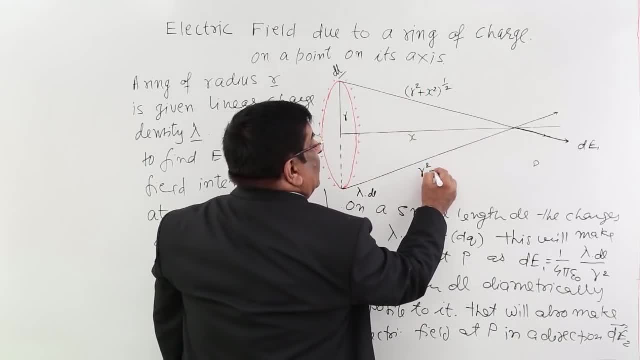 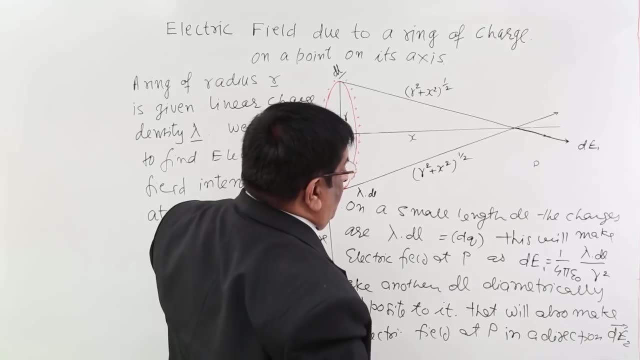 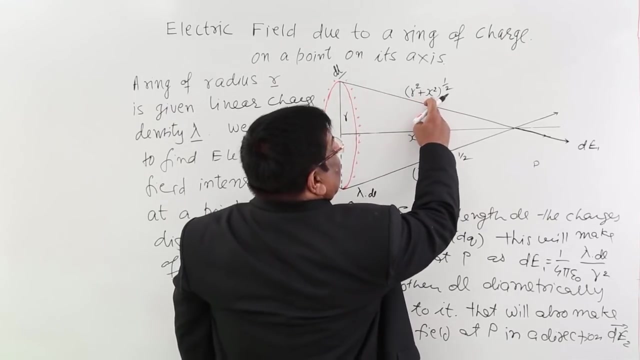 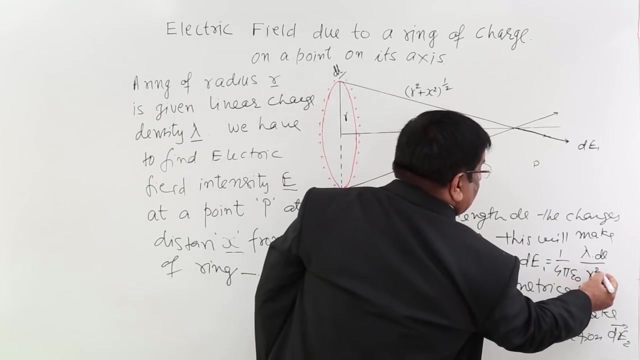 This is the same. So this distance is also same r square plus x square to the power of. Okay, Let me do certain correction here. Square of the distance: This distance is r square plus x square. So this, I should write it square of this, And how much square of this r square? 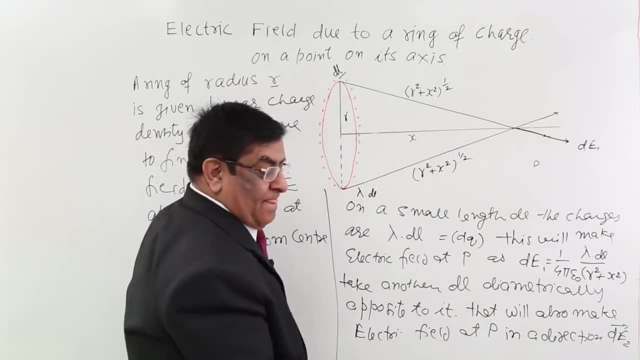 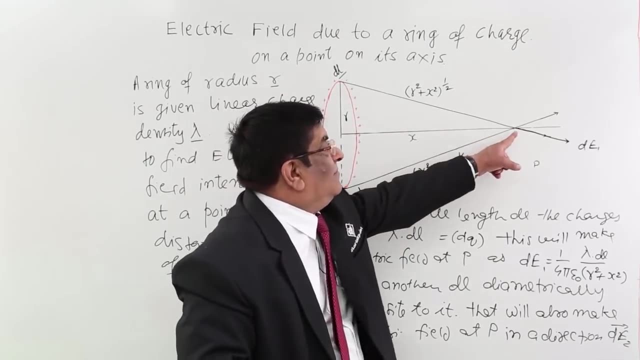 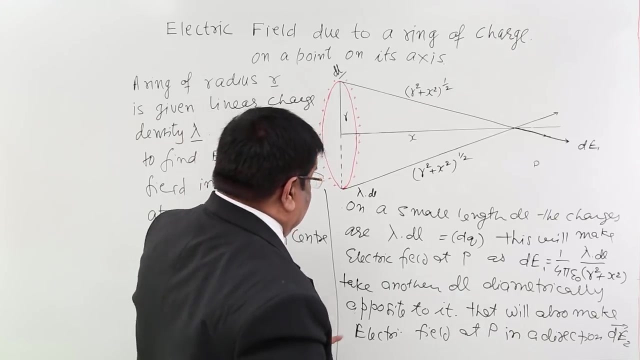 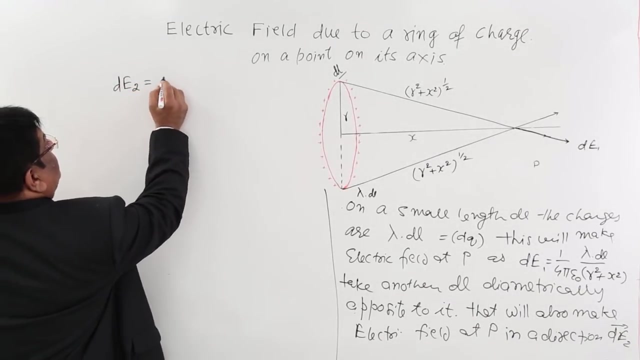 plus x square. yes, Eul, Eul. that was for this dL. Now what is electric field created by this lambda dL? Same distance, so this will also be same. So I will write it: dE2, same quantity, that is dE2, dE2 is equal. 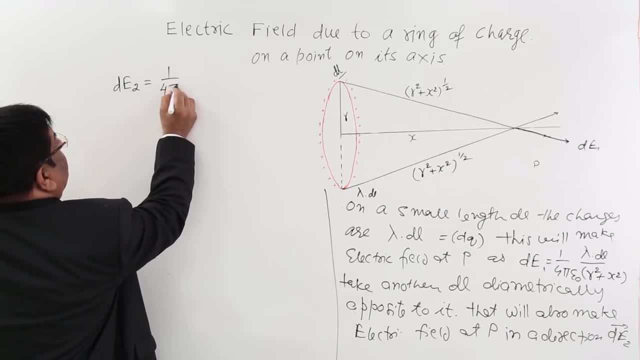 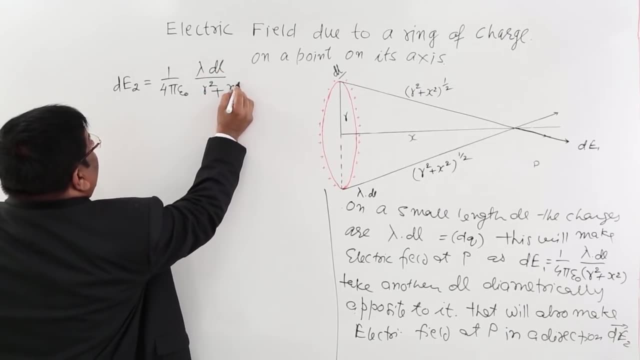 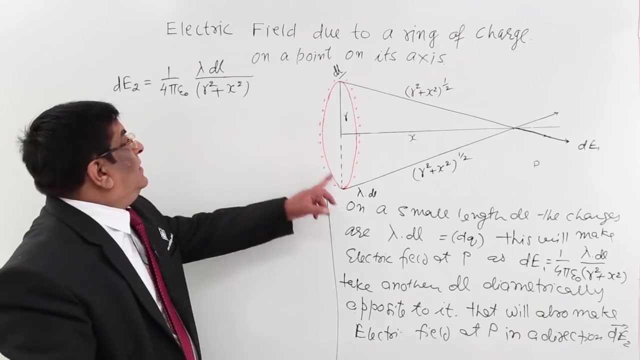 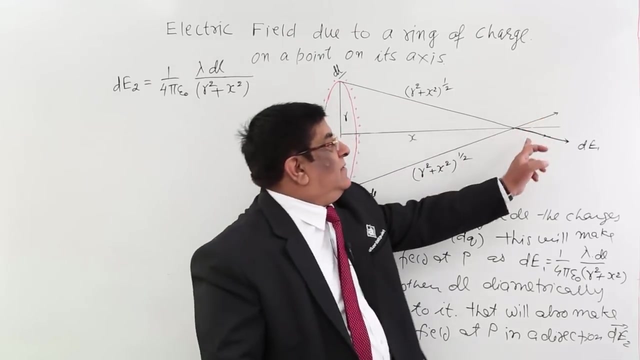 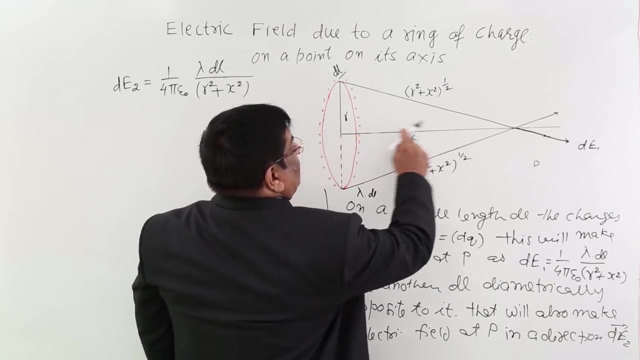 to 1 upon 4 pi epsilon 0 here lambda dL upon R square plus x square. So now you see, the magnitude of 2 are same, but directions are different. Another thing we can make out because of this symmetry: R and x, R and x. if this angle is taken as theta, this also can be taken as theta, this: 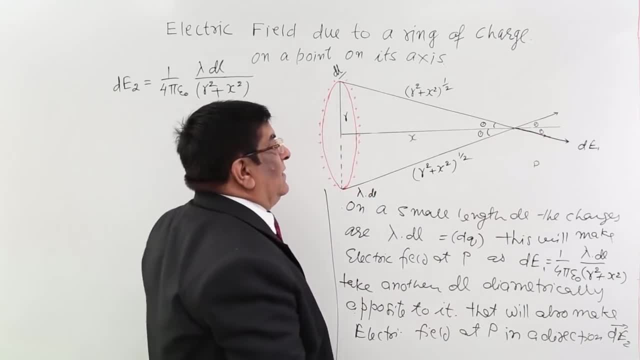 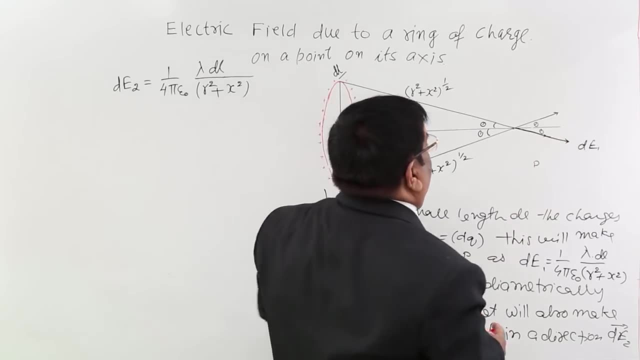 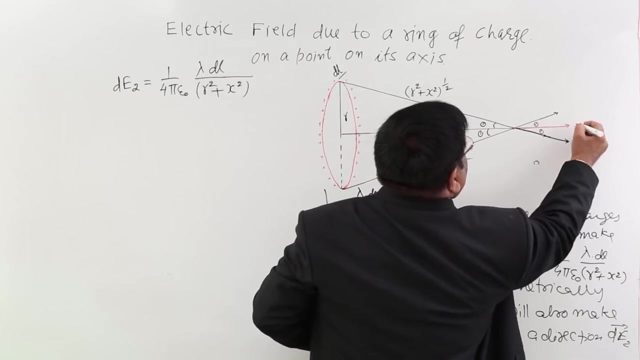 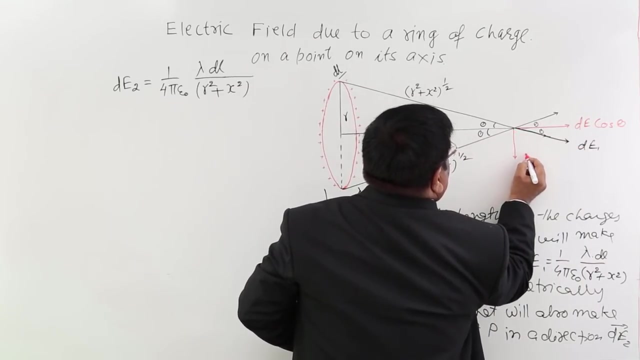 is theta, this is theta. Now, this electric field dE1 will resolved into 2 components. One is along the axis, that is this: how much will be this component? dE Cos, theta, cos, theta. That is this theta and this will be dE sin theta. Similarly, for this electric field, we have two components. 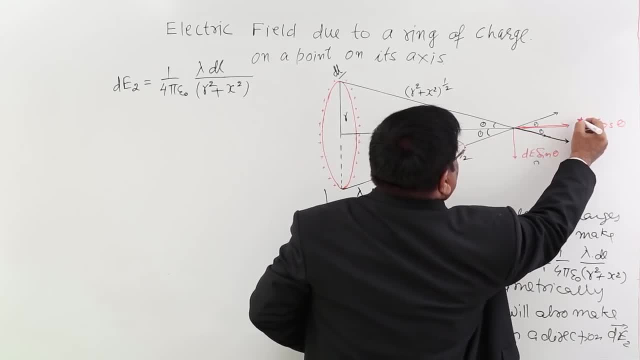 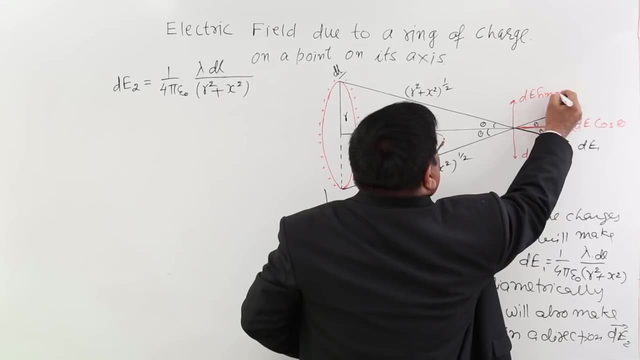 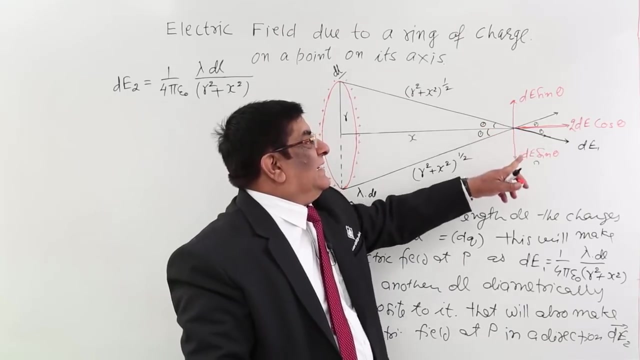 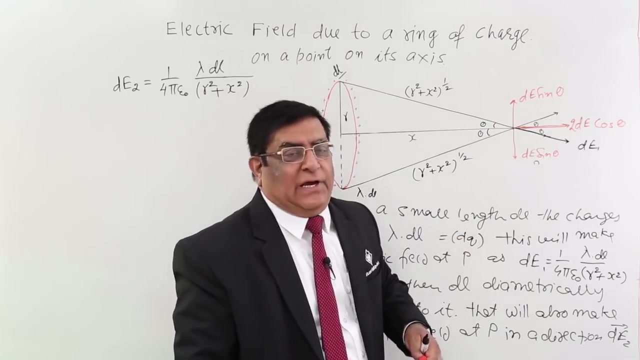 one is along the axis, that is dE cos theta, and this is dE sin theta. and now this is very clear to you: dE sin theta component of these two will get cancelled and we get resultant electric field in the direction of axis that is 2 dE cos theta. This is when we have taken 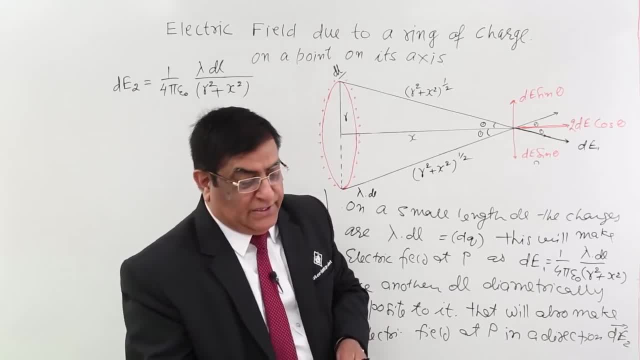 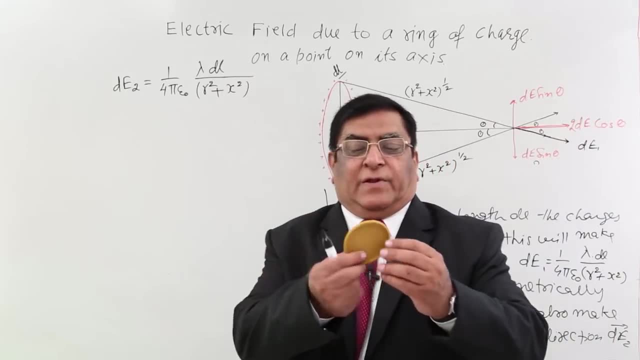 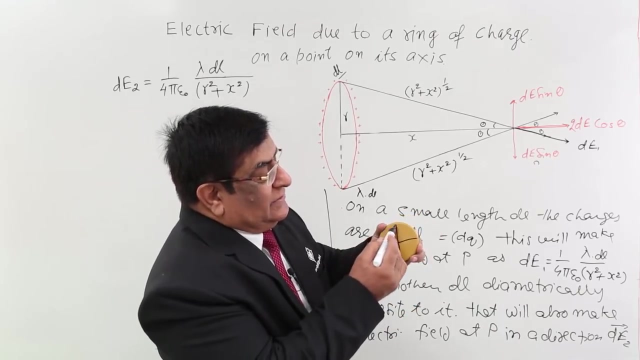 two points diametrically opposite. Now, when we take two points diametrically opposite, we have another diameter also, and that diameter is: if this is one diameter, then this is another diameter. These two points- dL, dL have given dE cos theta, dE cos theta, these two points this will make. 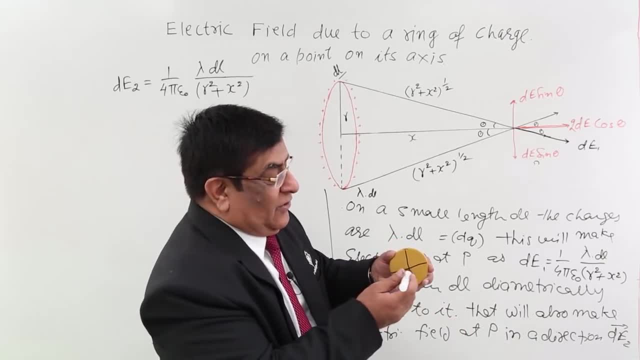 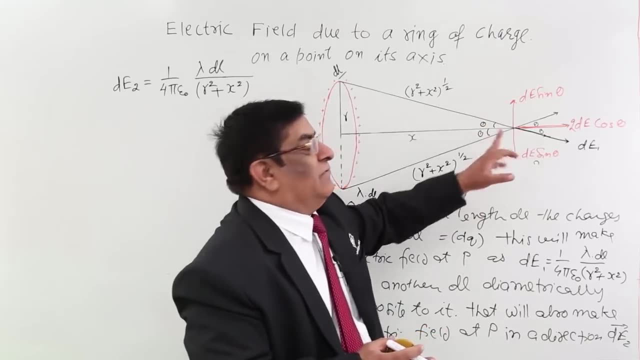 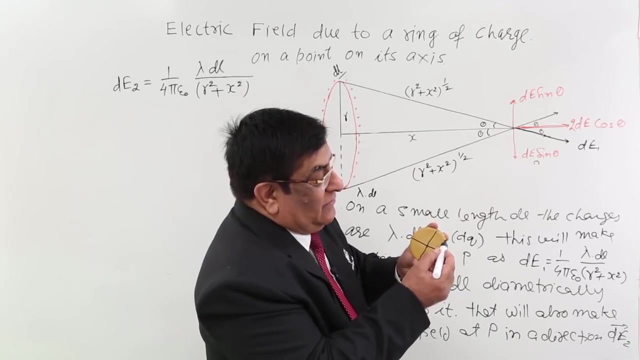 electric field here. this will make electric field here for them also. dE cos theta and dE cos theta will be the remaining one. dE sin theta will be cancelled. So for every electric field, dE sin theta of this point will be cancelled by dE sin theta. 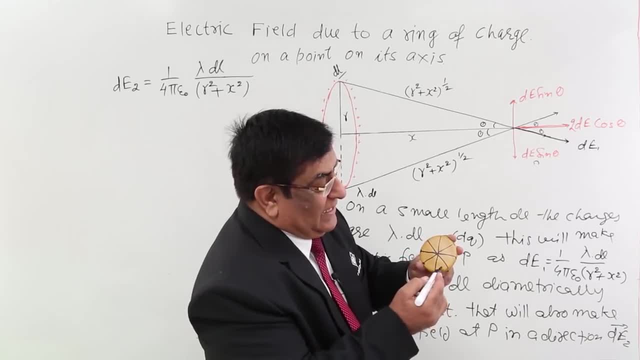 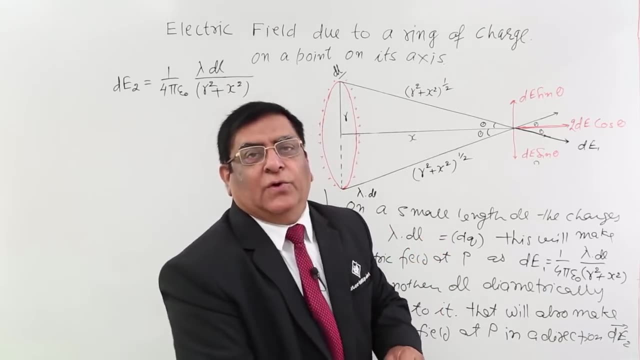 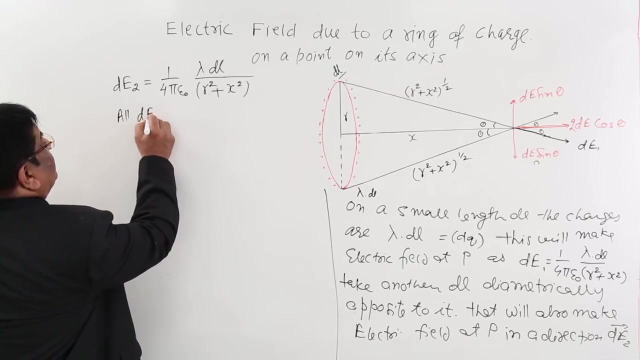 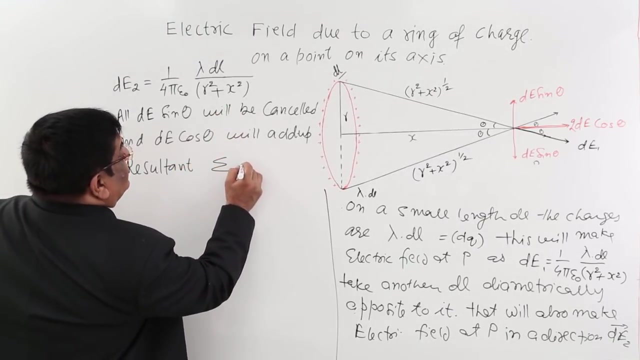 Of this point, dE sin theta of this point will be cancelled by dE cos sin theta. of this point, all dE sin theta will be cancelled. So what will be the resultant electric field? I will write the same thing: all dE sin theta resultant will be sigma of dE cos theta. Okay, now how. 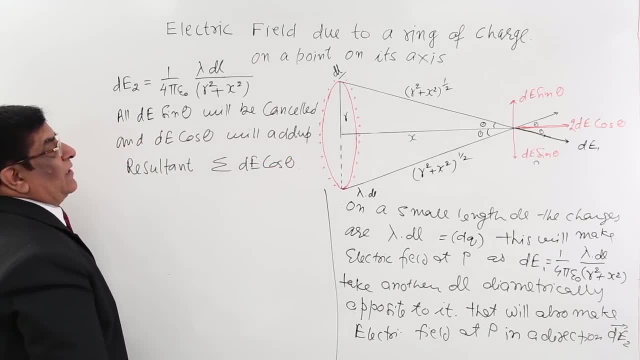 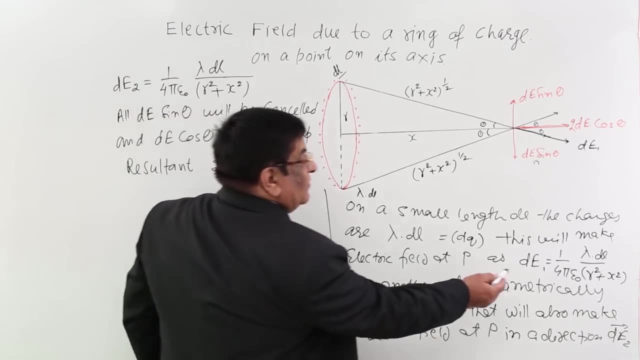 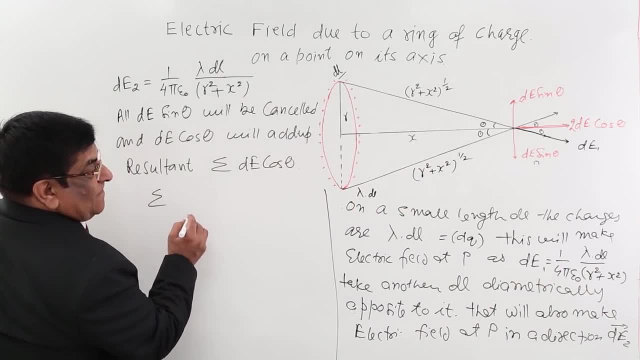 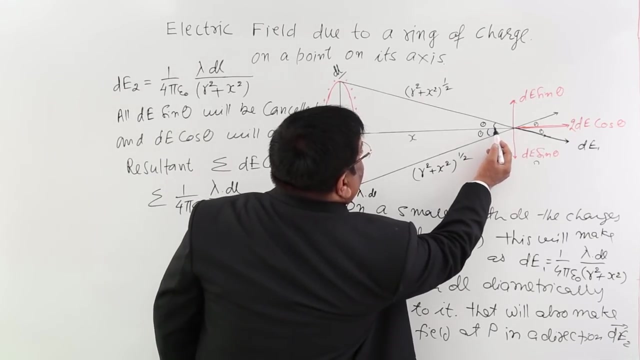 well write it. So this is sigma of 1 upon 4 pi, epsilon 0.. This is lambda dl upon R square plus x square multiplied by cos theta. Now, if this is theta, this is theta. I can always find out cos theta by trigonometry. that is base upon hypotenuse. So this is base, this. 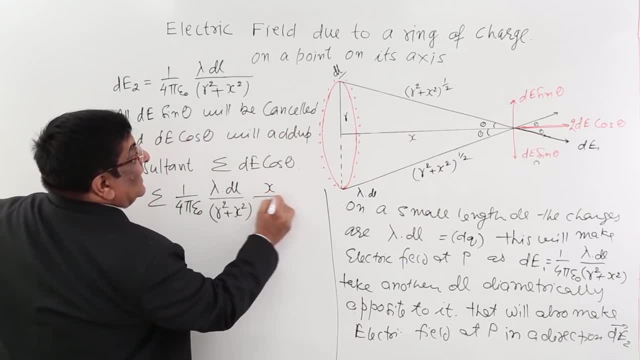 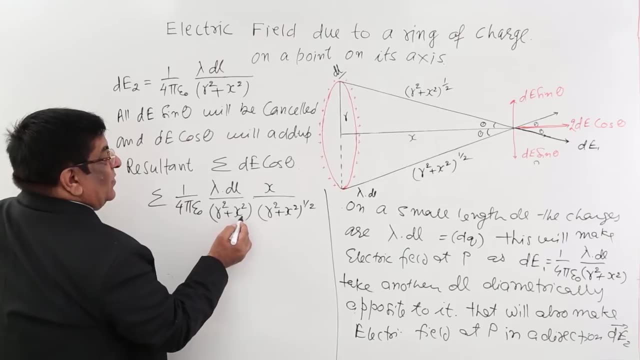 is hypotenuse and cos theta I can write as x upon R square plus x square to the power half. Now, here R square plus x square has power 1. Here it has got power half, so both will be added up. this will be R square plus x square. 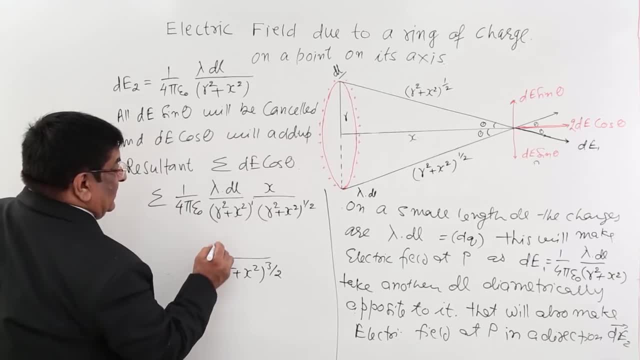 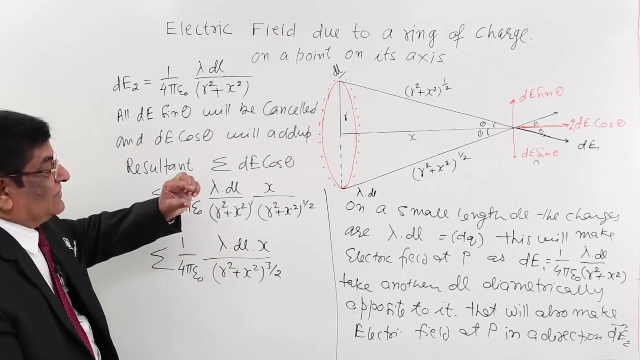 to the power 3 by 2. And here we have lambda dl x 1 upon 4, pi, epsilon 0 sigma. Now if we take very small, this dl, which is tending to 0. And we have to take all the dl, then this sigma means integration, adding up all the. 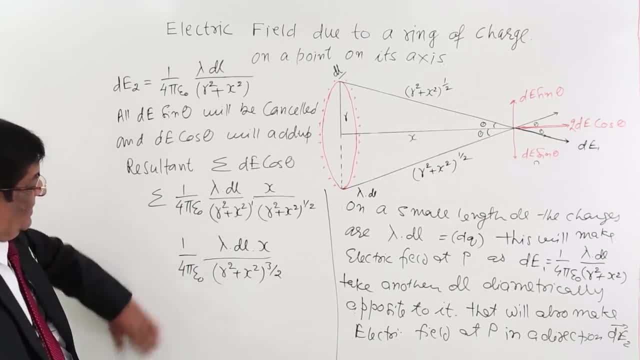 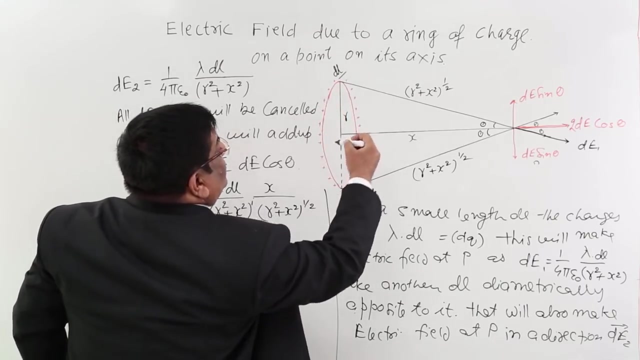 dl that means integration. So this we can very well convert to integration for complete circle. So closed integral of dl is the total length. this and how much is the total length? If this is the radius R, the total length is 2 pi R. So now this is the total length of dL over L and that. will be 1 over r. What we are going to do in the next class is this: In the next class we are going to solve the problem that if I divide this into 2 pi R by 2 pi R, So here: 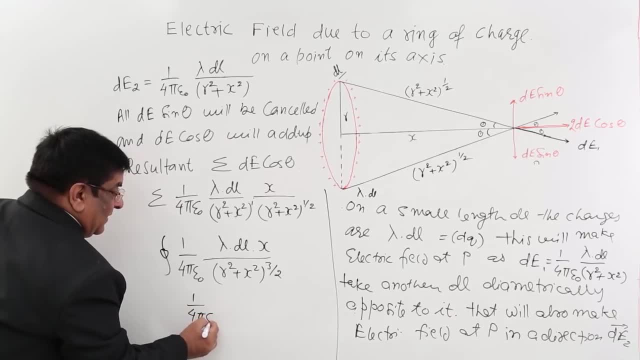 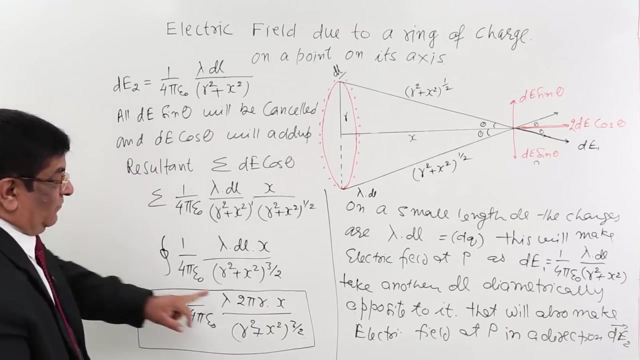 we can write it 1 upon 4 pi, epsilon 0, this is lambda- into 2 pi r, into x divided by r square plus x square to the power 3 by 2.. Now this is our expression for electric field due to ring at distance x. It will be like this: This 2 pi r is what The total length. 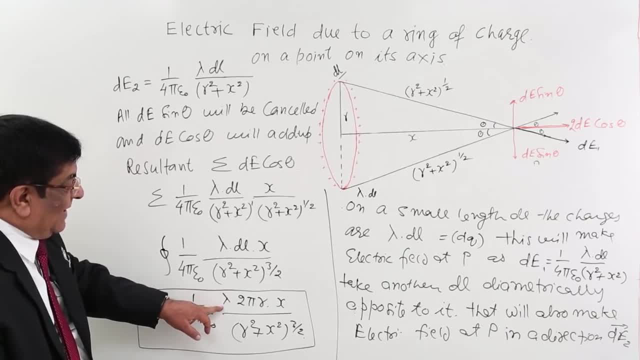 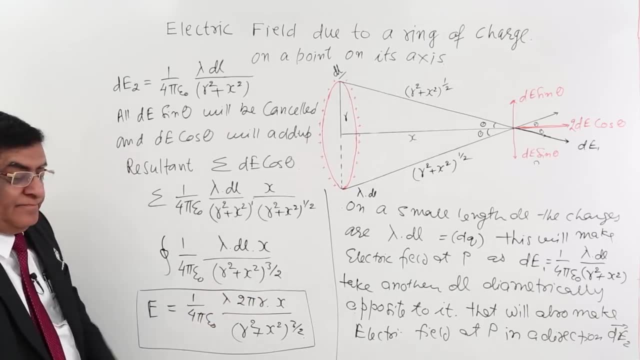 The total length. lambda into total length. Lambda into total length is charge q, So we can very well replace it with charge q. That can be done. We can write it lambda 2 pi r or, if we want, we can make it charge q. 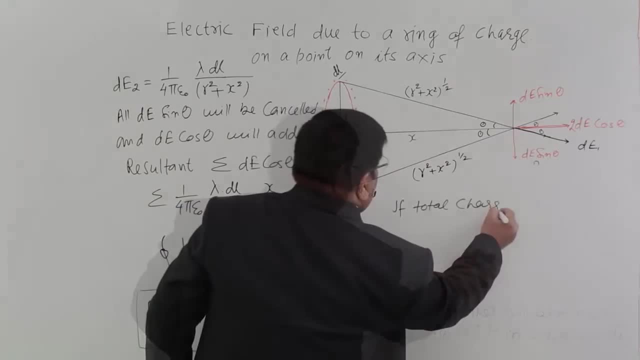 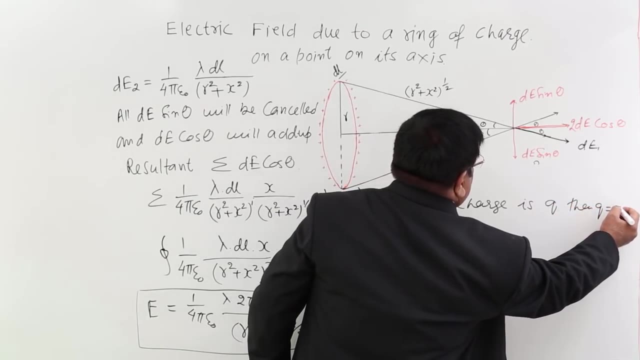 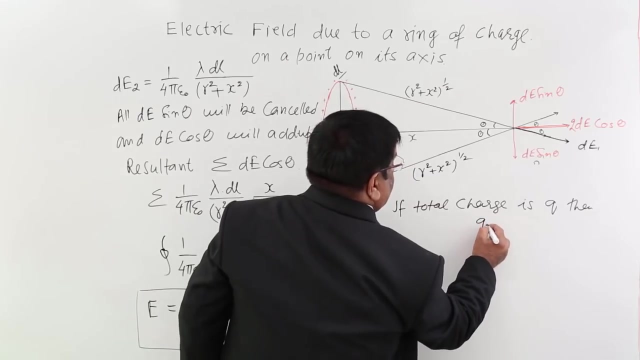 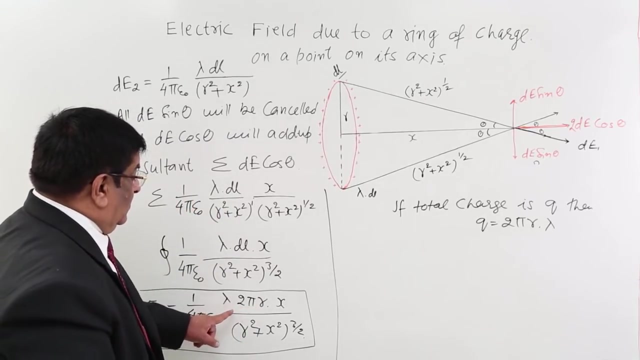 In that case this will become simpler. Total charge is q. Then q is equal to 2 pi r into lambda. or I will write it: q is equal to 2 pi r into lambda. This 2 pi r into lambda, ok. Another thing: ok. 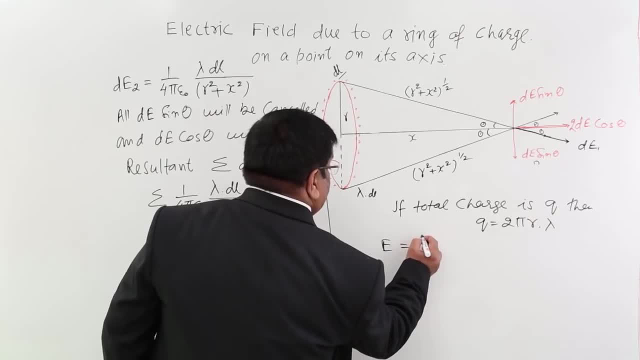 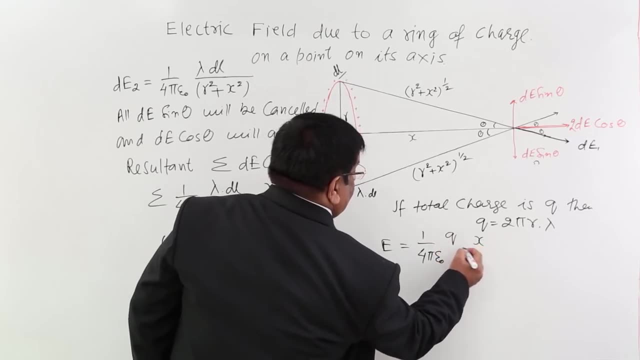 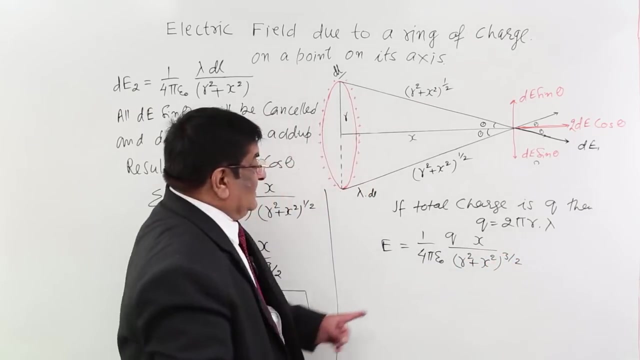 So this way will be: electric field is equal to 1 upon 4 pi, epsilon 0, here Q x upon R square plus x square to the power 3 by 2. This is constant of the medium, this is charge and this is. 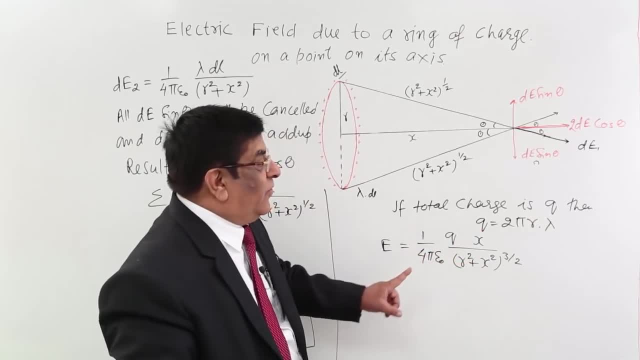 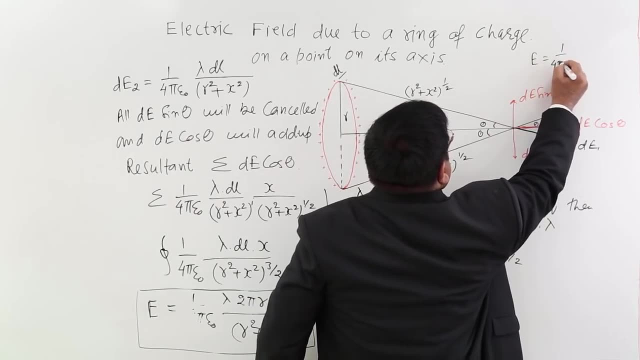 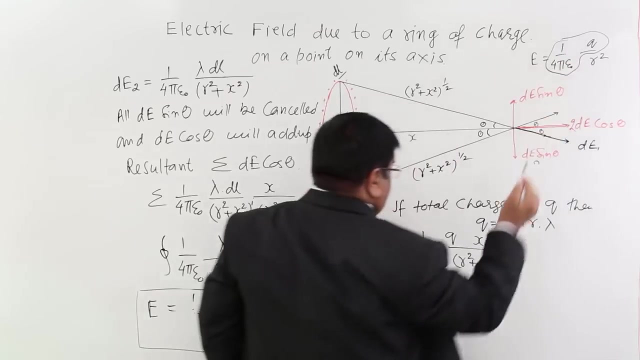 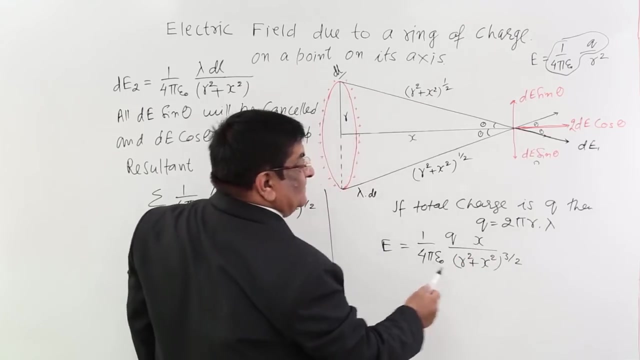 all the distances which matters. General formula for the point charge. what do you know? The general formula for point charge is: 1 upon 4 pi, epsilon 0. Q upon R square: 1 upon 4 pi- epsilon 0- Q. it is there This much. In place of 1 upon R square, we have this formula. 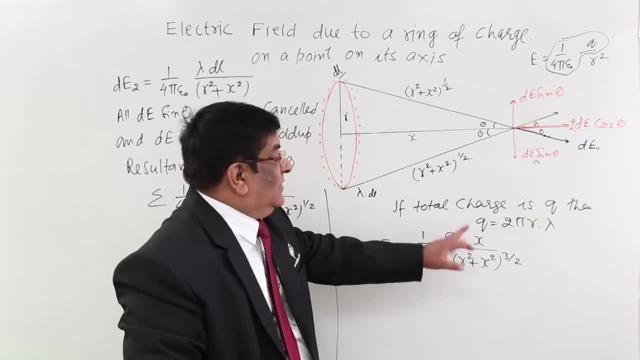 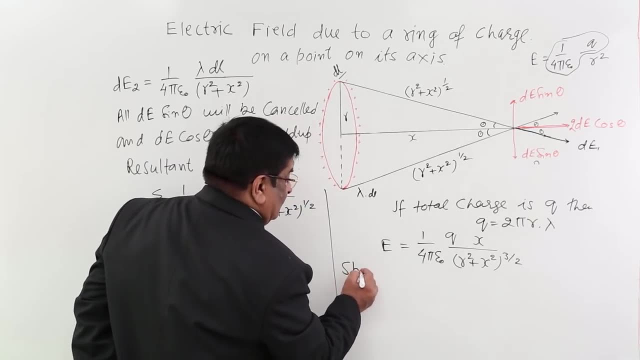 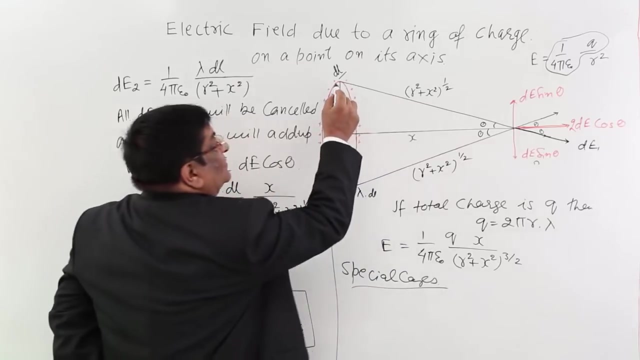 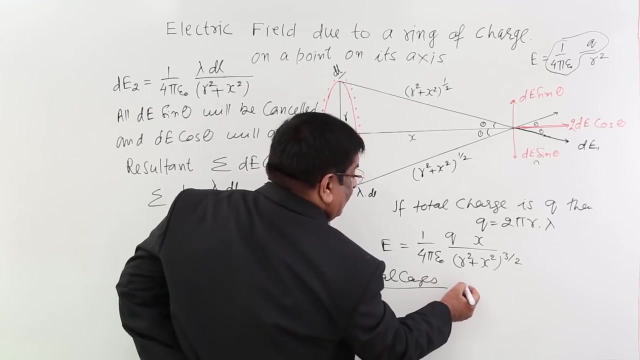 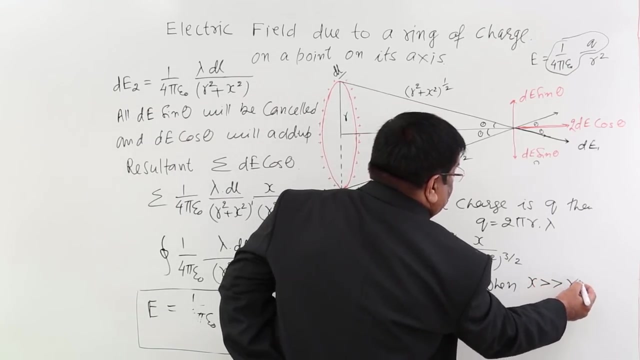 So when x increases, this goes on decreasing, Why x has got more power here. Now we take the special cases. Special cases means if this X is very large compared to R, then we will neglect R in this addition And this formula number 1, when X is very large, then R If X is very large. 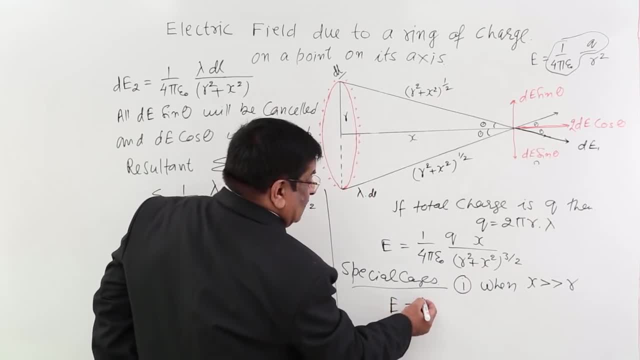 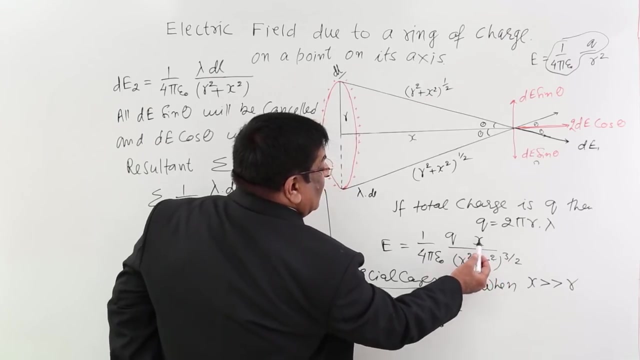 than R, then E is equal to 1 upon 4, pi, epsilon 0. Q upon This is neglected. X to the power 2, 2 to the power. 3 by 2 is equal to X to the power 3 and 1. X is cancelled. What we 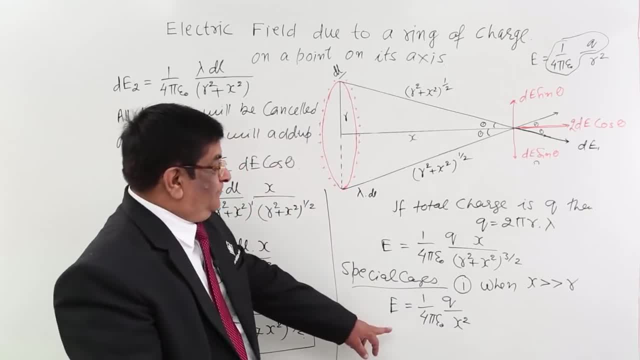 get here Q upon X square. Now compare it with this point charge. So when the distance is 0,, then point charge is 0.. So when the distance is 0,, then point charge is 0.. So when the distance is 0,, then point charge is 0.. So when the distance is 0,, then point. 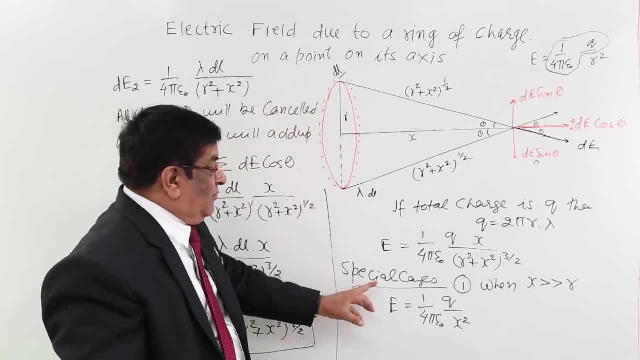 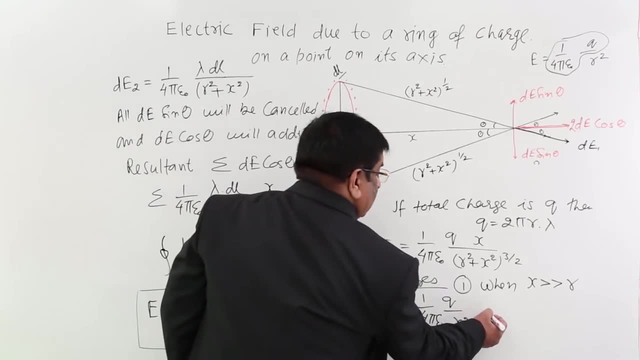 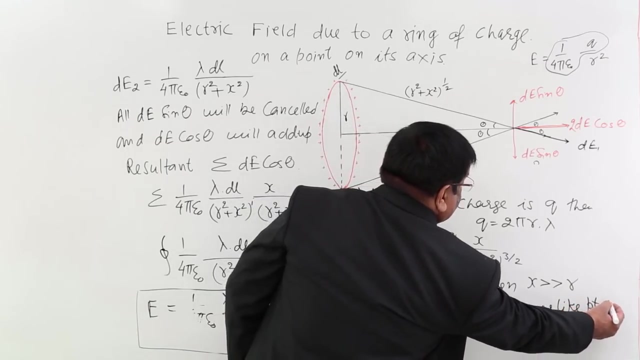 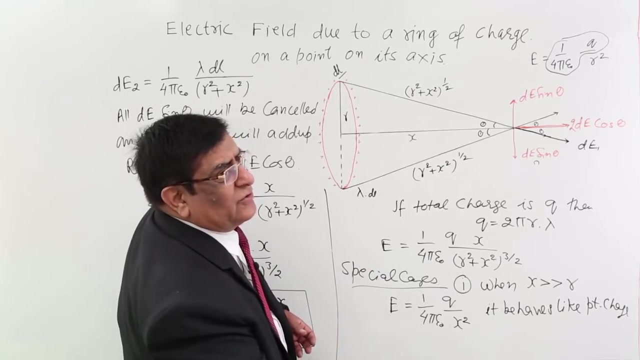 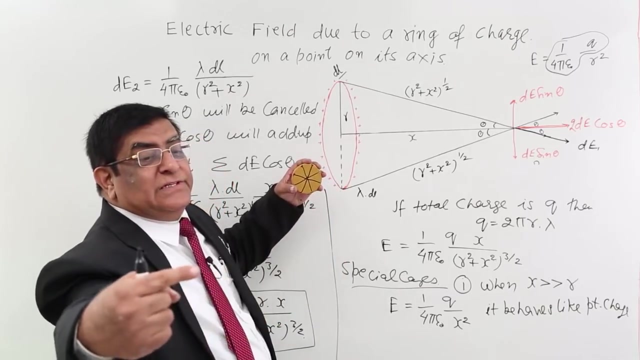 is very large, this whole ring will act as a point charge. This distance is x, so this is 1 upon x square. It behaves like point charge. Okay, And that is very clear. also, If you have a ring over here for this, this will be different. But if you go to this much, 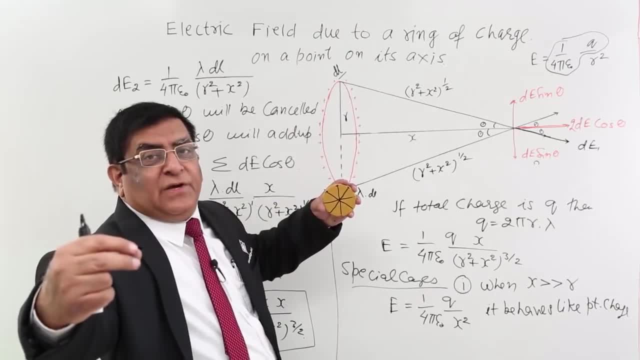 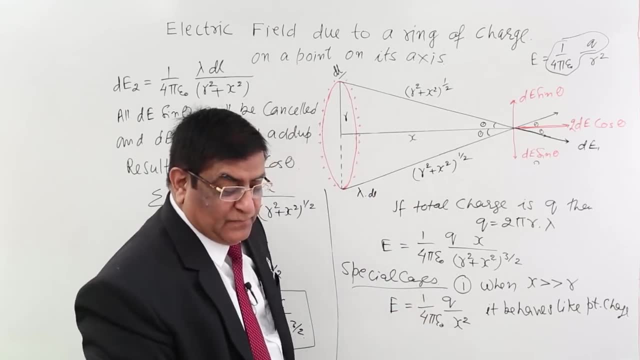 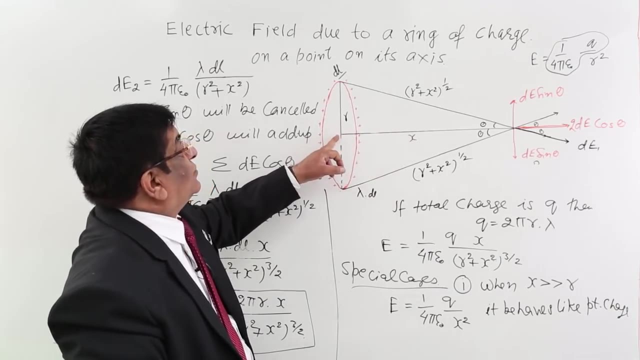 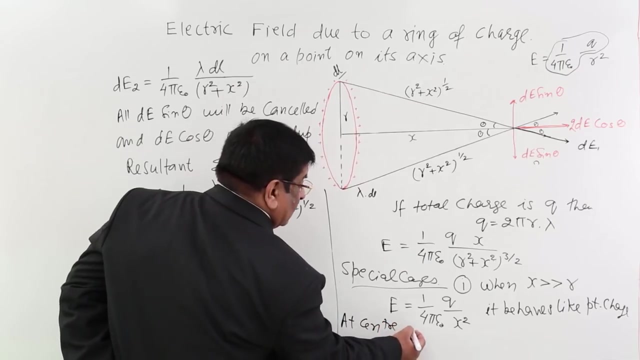 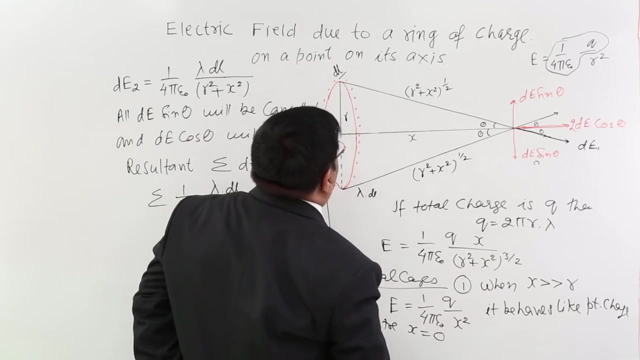 distance, then almost theta becomes so small that all the lines appear to be parallel. So it behaves like this: Now, if x is very small, this much, this much, this much- and comes to the centre, That means at centre, center, x is equal to 0. If, at center, x is equal to 0,, then this will be effective. If